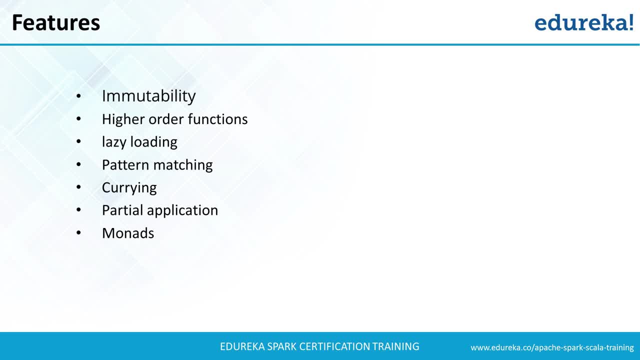 And the first property is immutability. so we have already seen immutability. So any functional programming will have these seven properties. So firstly, immutability is there, which we already saw. how we achieve immutability through the val keyword. 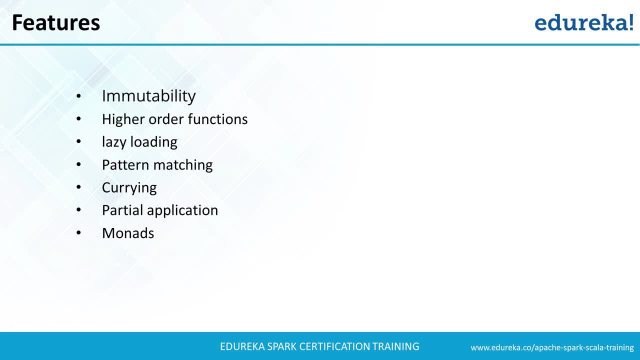 Then it supports something called higher order functions, So higher order functions, which we are going to learn today, so it's going to have higher order functions. And then it supports lazy loading And lazy loading. we have already seen lazy loading. We have already seen immutability. 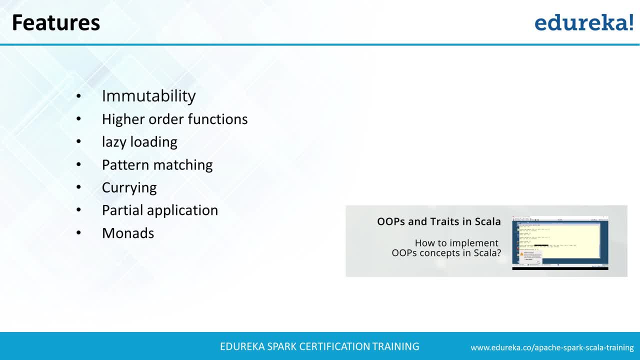 We are going to learn about higher order functions today. So that's about the three things, but there are four more things, which basically makes You know functional programming what they are. There's something called pattern matching, curring. This is not the Indian or the Thai curry. 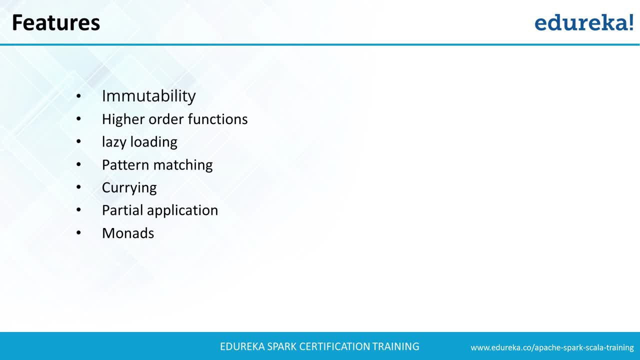 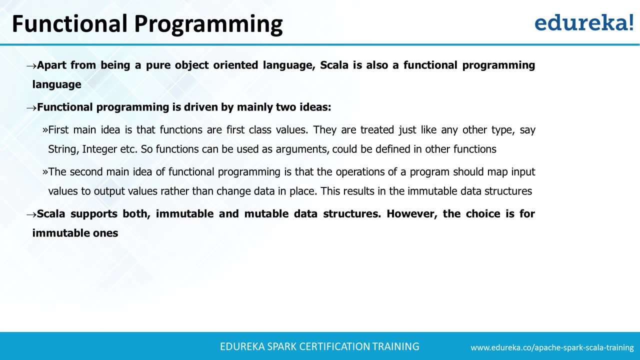 This is a mathematics concept called function curring, And then you have something called partial applications and then something called monads. So all these seven properties actually goes into make. Okay, so let's learn higher order functions and functional programming. So let's look at what functional programming is all about. 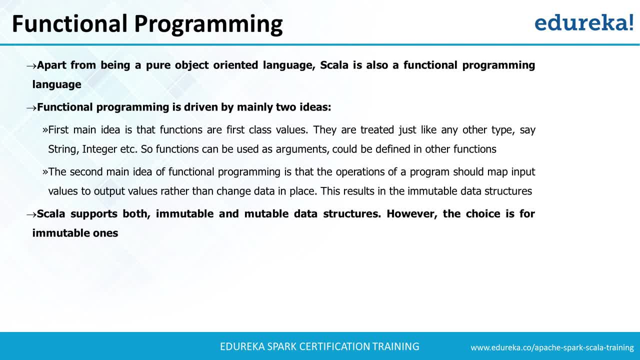 I told you about So far. we saw the object-oriented aspects. Now we are going to see the functional aspects of it. So first of all, let's look at the functional aspects. So firstly, we saw that functional programming is mainly based on two ideas. 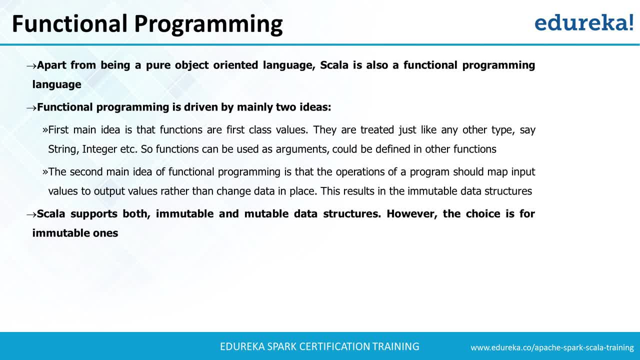 The first thing is that functions are first-class citizens. So what do you mean by functions are first-class citizens? Functions are first-class citizens because it means that you can treat the function just as any other variable. So let's prove it. So here I am in this color prompt. 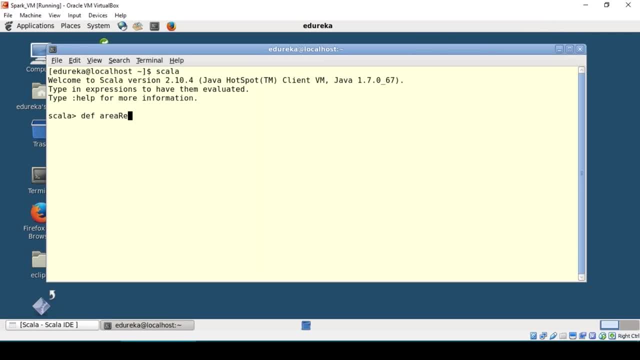 So here let me write the area, our old area function length, into here. Let's keep it simple. So here I have defined a function. Now I can call areaRect like this: So it prints 90. Now what I can do is I can define a function f, a variable f and I can assign the function to any variable. 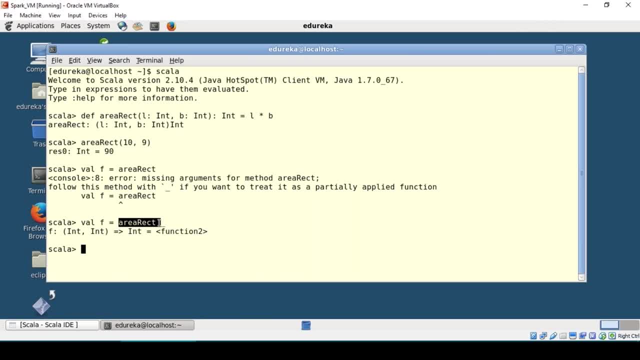 So basically this function, areaRect, just behaves like a variable, So I can assign this function to another variable and then I can call f just like another function, So it will print 90. And if you print the signature of f it basically completes. 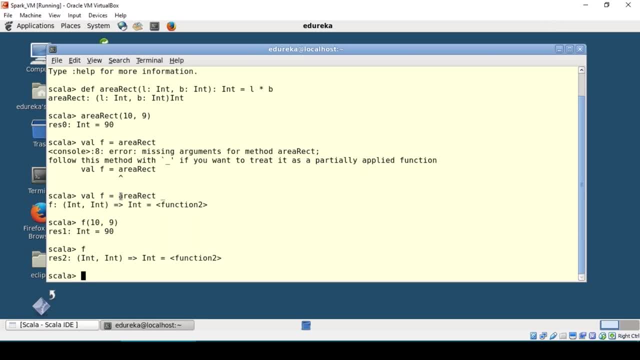 It basically complies to the signature of rect. So here we have proved that a function basically just acts as a first-class citizen, because it just acts as any other variable. You can assign it to variables And you must have noticed this underscore which I have put after this areaRect. 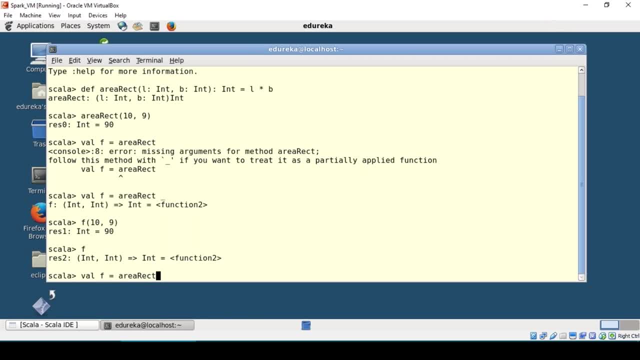 So this is a Scala syntax. See, the thing is that if you just put areaRect, it will try to call the function. So the compiler is going to the runtime, is going to actually call the function. So that's why you see that it's trying to call the areaRect. 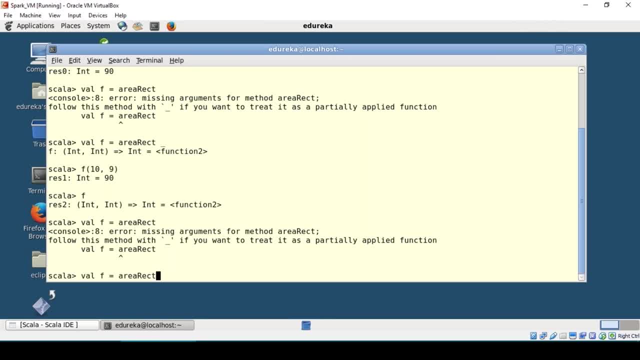 So here we don't want to call it, We just want to assign the reference of areaRect to f. So that's why we give an underscore. So an underscore here in Scala basically means that after a function name it means that I'm assigning the reference to it. 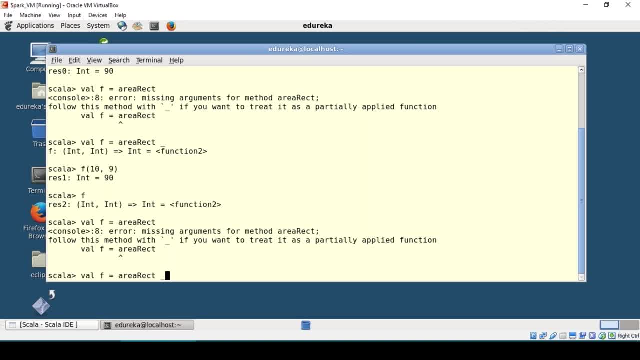 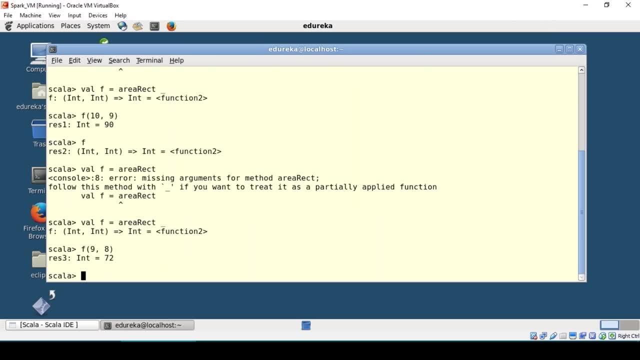 I'm not calling the function, So the reference of areaRect and the address of areaRect is assigned to f, And then I can call f like any other function. So it's not a lazy call, Ganesh, It's not a lazy call. 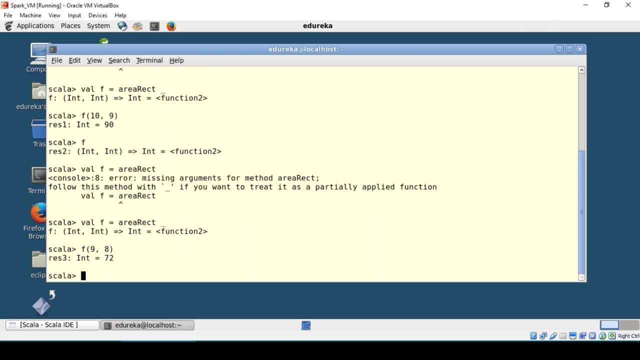 It's basically just an assignment. That's how you assign functions. So we have proved that It can be just treated like a variable and it can be assigned to another variable. Now we are going to prove that it can be passed around just like any other variables and it can be also returned from functions as variables. 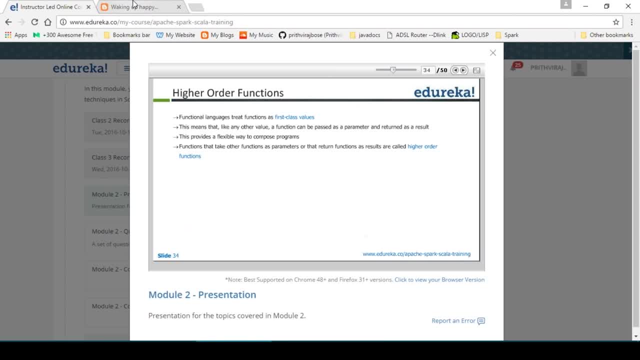 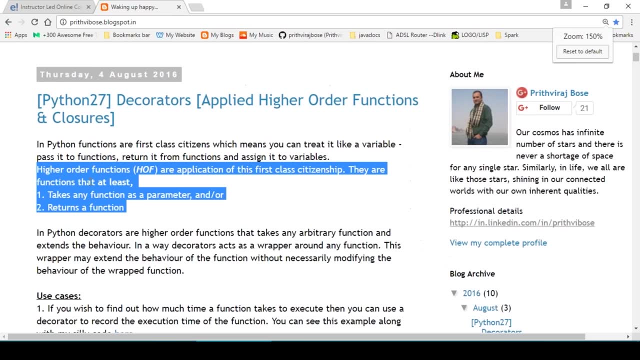 So these are basically first-class citizens. And now let's see what higher-order functions are. So just remember this particular principle of higher-order functions. So basically, higher-order functions are applications of first-class citizenship. They are any function Which does at least any of the two. 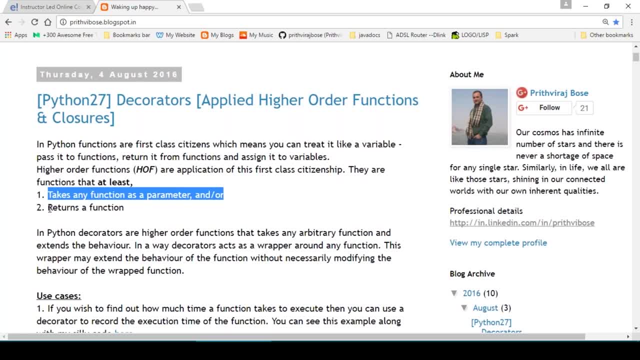 So it takes any function as a parameter and or returns a function. So if any function takes another function as a parameter or returns a function as a return value, then it becomes a higher-order function. So just remember that your functions are first-class citizens. 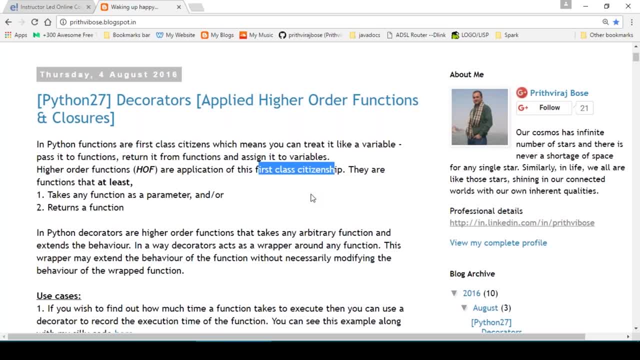 And by first-class citizens I mean that they can be treated as any other variable And higher-order functions are functions which does at least one of the two. That means it takes a function as a parameter and or returns a function. Clear all of you. 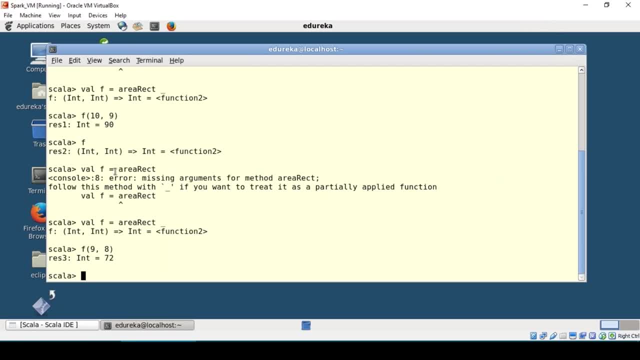 What higher-order functions are, What first-class citizenship is. So here I showed you what first-class citizenship is. Now I'm going to show you how we can pass functions as parameters. Any questions so far? So let's define a method called add, which takes integer a and integer b and it returns the addition of a plus b. 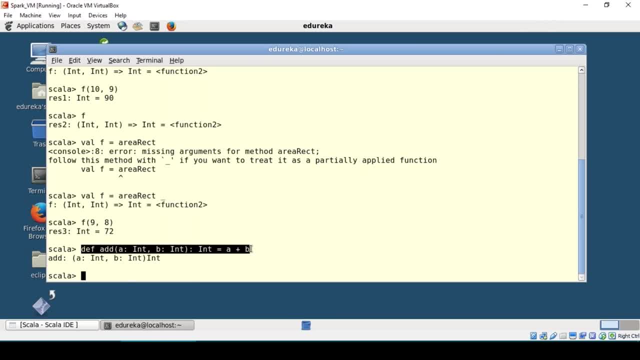 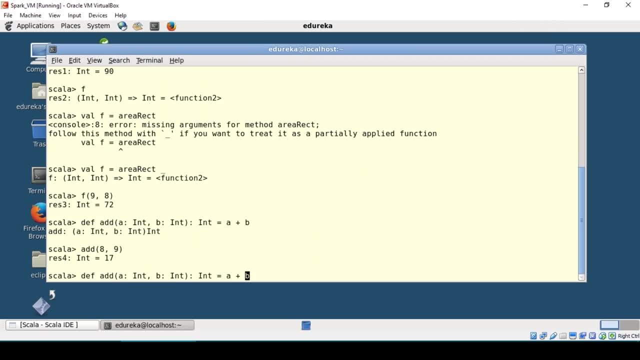 So this is the function I've written. So I defined a function- add- which takes two parameters: add. So this is just for example. So now I can pass 8 and 9, and it will give me 17.. So similarly, I can write another function called multiplication, which basically takes a and b and gives us the product. 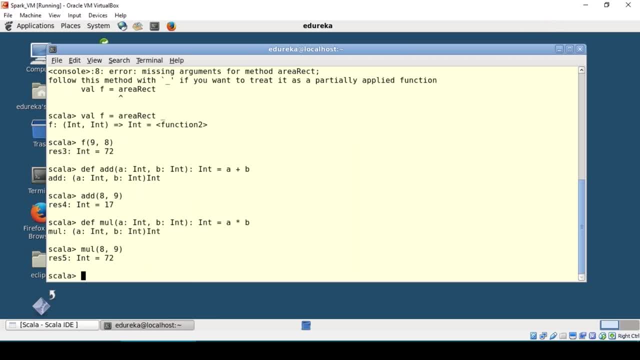 So 8,, 9, z will be 72.. So these are the two functions we have defined. Now let me write a generic function. So let's write a generic function f. What it's going to do, it's going to basically take. 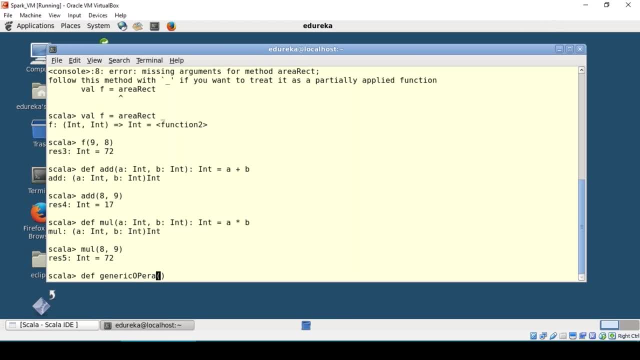 So I write a generic function or a generic operation Which basically takes a function First. tell me, I mean, are you clear with what I'm doing so far? this area, rect and these things. Do you have any doubts? If you have doubts, you can quickly ask me before I get into anything complex. 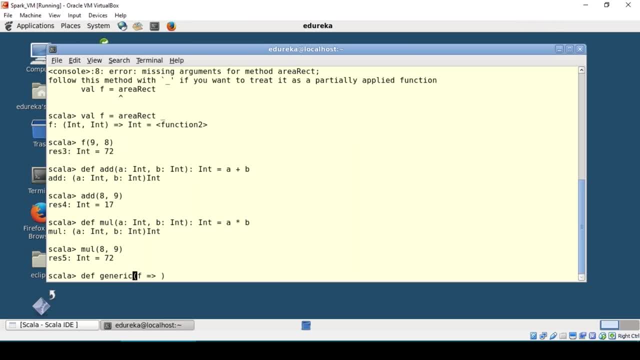 Okay, good. So now that you've understood, okay, Fair enough. So now what I do is I define something called a generic operation, where I define a function which, basically, will have two integers as parameters and will return an integer, And will return an integer. 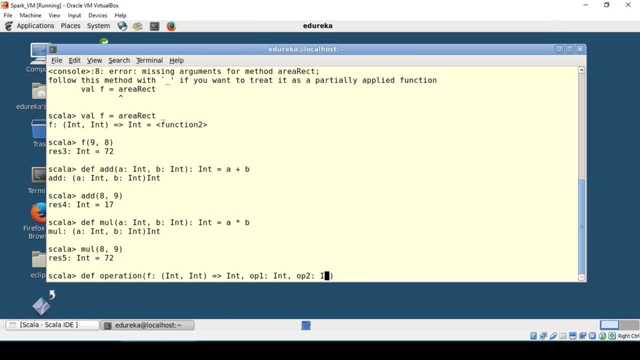 I give an operand 1 as integer and an operand 2 as integer, And this basically returns an integer. So did you understand this? Let's go through the syntax which I wrote. So here what I'm doing is I'm defining a function called operation, whose first parameter is basically a function. 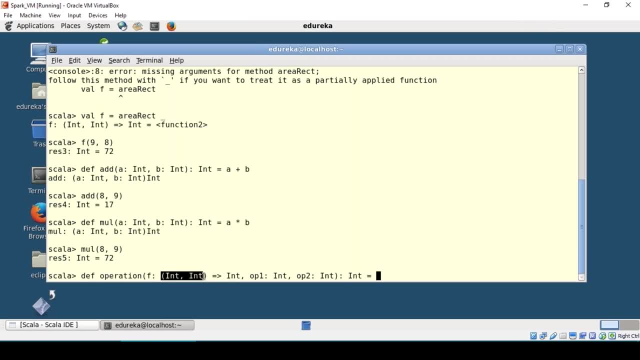 Its first parameter is a function And this function signature is that it takes two parameters and basically returns an integer. So it basically takes two integers as parameters and returns an integer. So that is a function I've defined here. If it can be anything, you know you can write ABC, anything here. 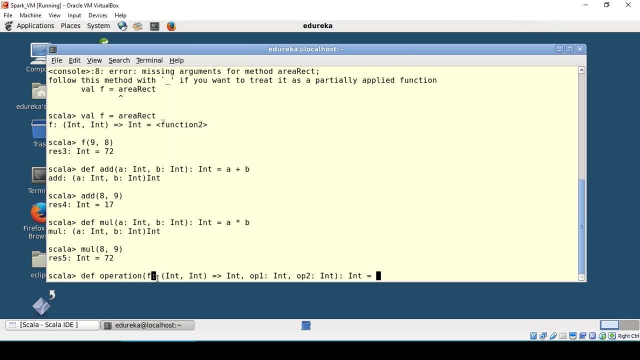 So, since it's a function, I wrote F here, So the signature, and then you write a colon and then you say the signature should be of type this: That means it takes two integer parameters and returns an integer. Okay, And then what I do is, you know, I take two operands. 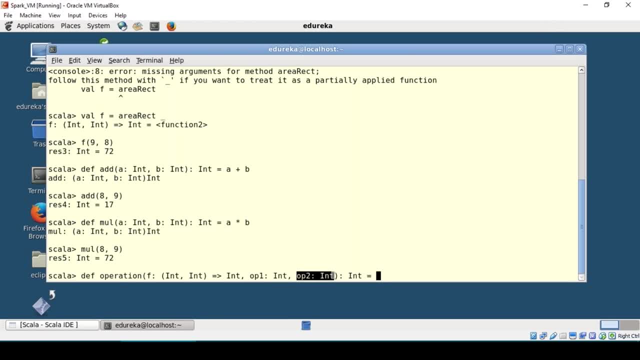 So I take the first operand as integer and second operand as an integer, And this function returns an integer, And in the body, what I do is this function. I call this function F, Whatever I'm passing here, as with the parameters OP1 and OP2.. 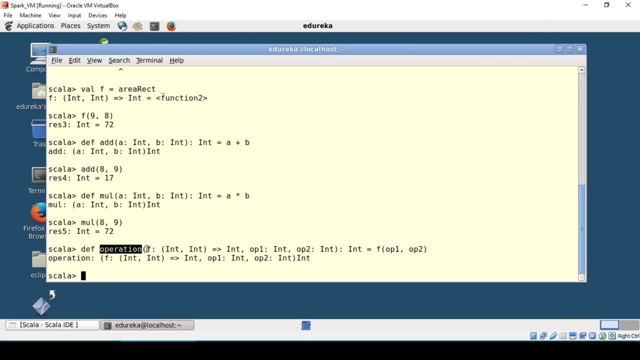 Okay, So that's the function I've defined. So it's a generic operation function where it takes another function of this signature and two operands. Okay, Now, what I can do is, you know, I can call this operation with add. Okay. 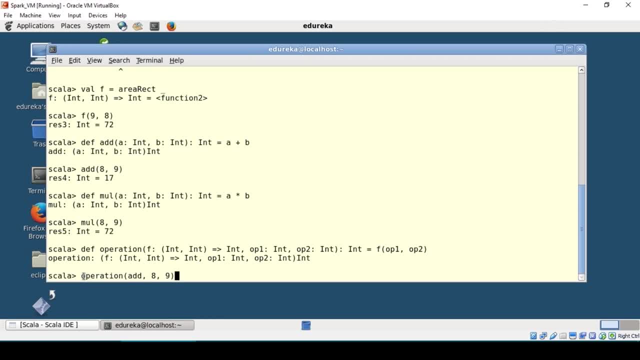 And I can call it a nine. So, basically, what I want is, you know, I want this operation function And I'm passing that function which I defined here. I'm passing the name of the function, add- And I'm passing the parameters which I want to pass to add. 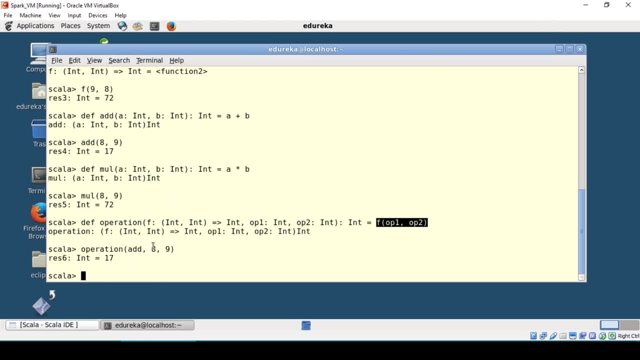 And if I call this internally, it's actually going to translate the call to add with these two parameters. Similarly, I can call in a multiplication, So I can give the name mal, which I defined here, And if I call this, it will print 72.. 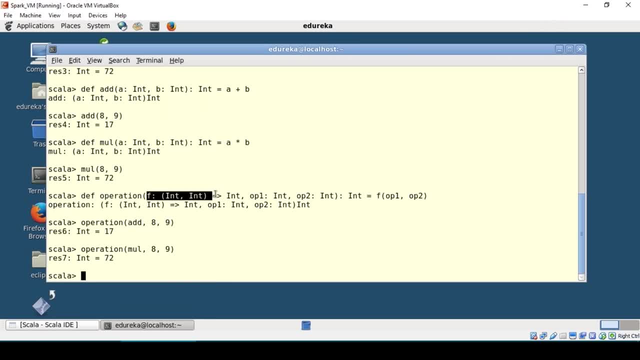 So that's how, basically, you know, we are trying to pass a function as a parameter And that's an application of add order functions. Did you all understand this? Any doubts you have? Just maybe look at the syntax and try to understand what I've done here. 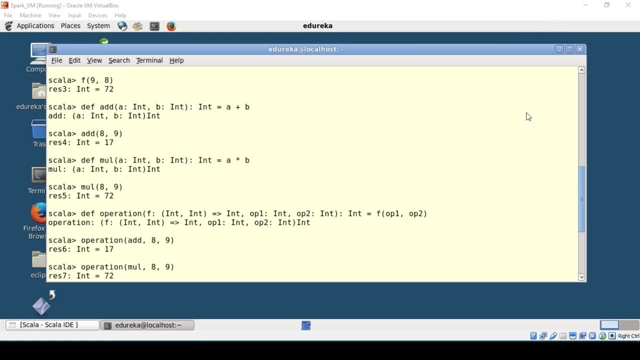 Okay, You, Rao is asking me, wants a couple of questions here. Ganesh is asking me. here. you call directly add function. Yes, you're right. So what I'm doing here, Ganesh and Praveen, is that I declare the generic operation. 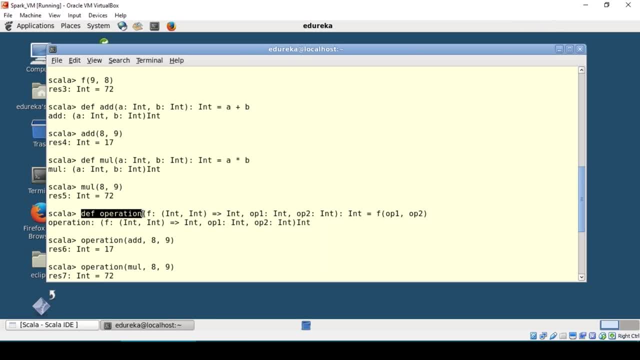 So, and what I can do is so here you know the generic operation. what I'm doing here is that you know I write the function declaration, Okay, And this basically has this particular signature, Okay, So that means that you know this particular. I have to pass any function. 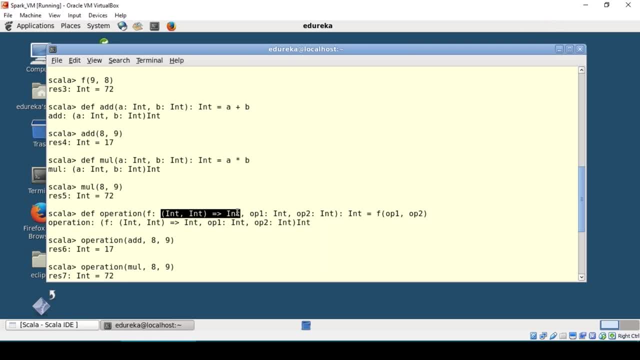 I pass any function which takes two integers as parameters and returns an integer. So as long as I pass any function which complies to this signature, this operation is going to work. And then I take the two operands which I'm going to pass it to this function f. 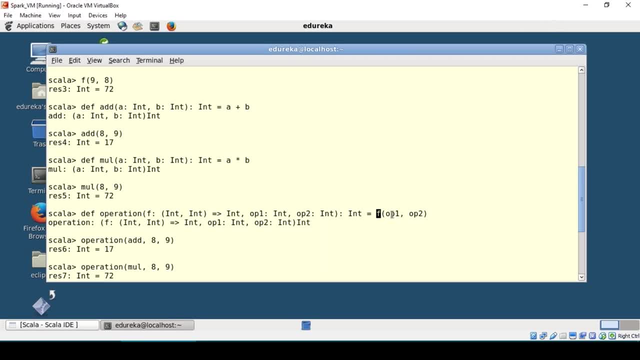 So in the body, basically I just call the f with the two operands. So it's generic kind of binary operations where you can handle multiplication, addition, anything Clear Praveen. Okay, Shailaja is asking me what happens if add and multiply were returning float and also defining returning float. 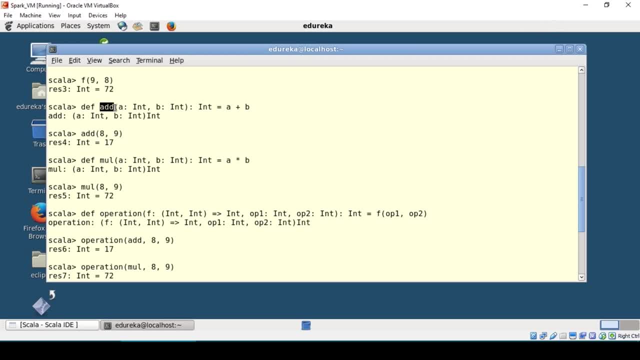 See, then you have to also define. you know, redefine, add and multiply to redefine float. So the best way is actually, you know if you can write a generic type. So instead of hardcoding the variable, you can write t here. 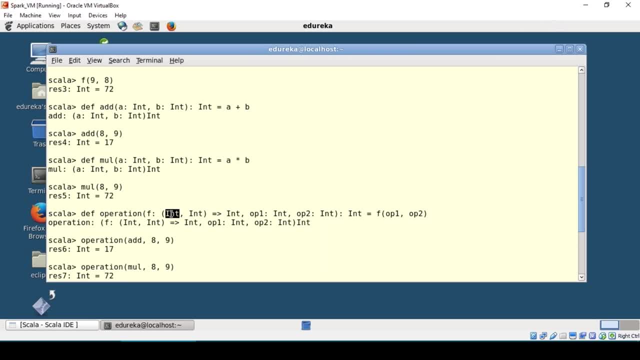 And you know I'll get to that a little later, Shailaja. First let's understand this basic thing, Okay, So I'll come to that a little later- how we can convert that to a generic type, Okay. 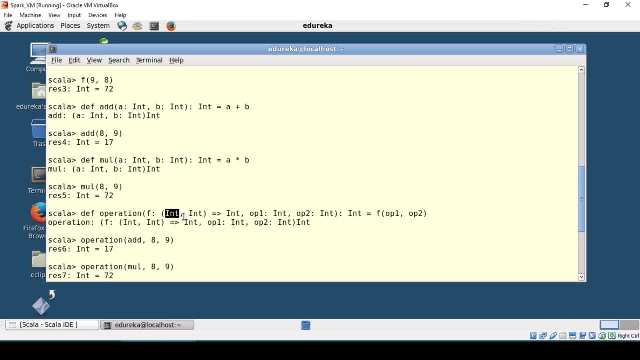 Vimla is asking me: can you pass any function implementation to f as long as they follow the f signature Right? Absolutely, Vimla. So you can pass any function you know, which basically takes two integers, Which basically takes this signature form. 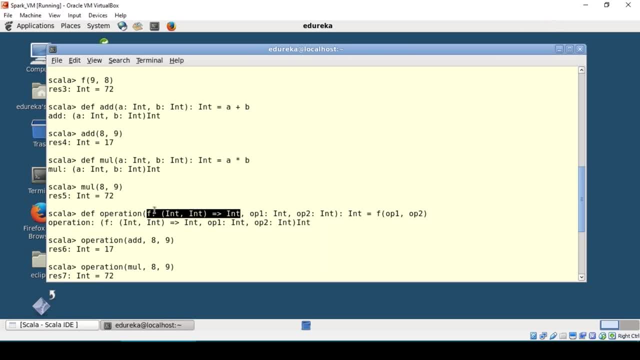 So that is also possible. Okay, The thing is that, Praveen, I'm just trying to explain to you the concept. you know, try to understand the concept first, because then I'll come to complex examples a little later. It is true that you know I can directly call the add and multiply. 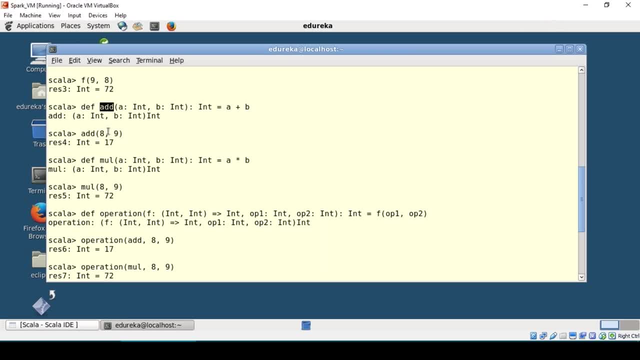 What is the big deal in calling through an operation? Many of you are wondering that I can directly call add and directly call multiply. So what is the big deal in actually, you know, calling it through operation? Well, this example may be silly. 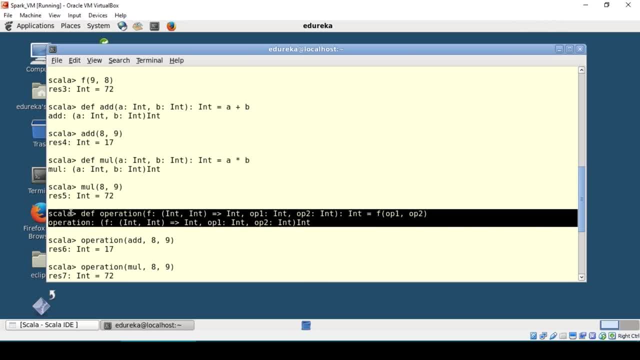 But what I'm trying to show you is actually how to do this. Once you've understood how to do this, then we can actually go to more practical examples which can keep your head scratching. So first try to understand, okay, what the stuff is. 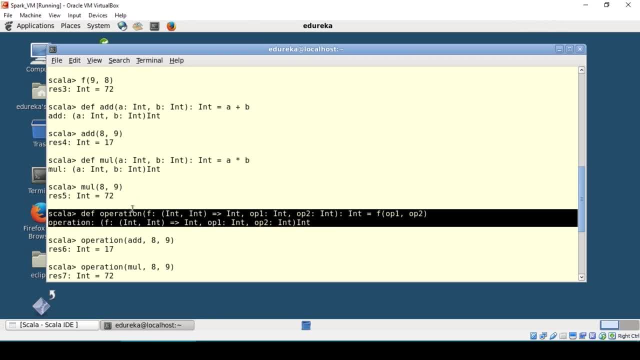 And then I'll actually give you a lot of practical examples, But try to understand exactly how the principle in principle, how it is working. Okay, My friends from Philippines, are you all clear with this? Rafaela, Kevin Erwin, Nona, Rina- yes, 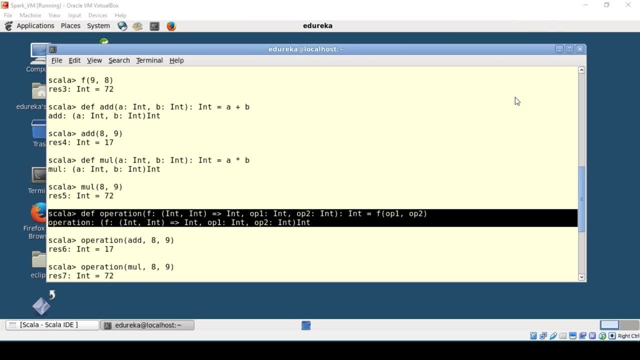 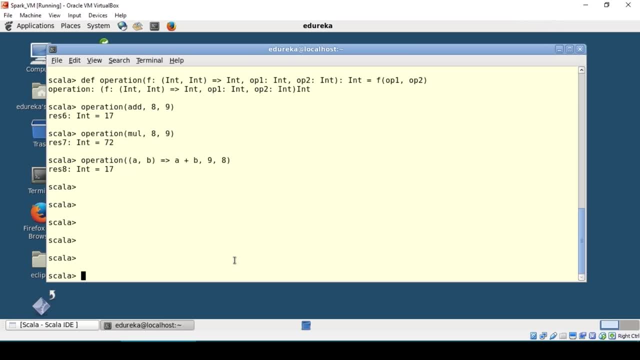 Okay, Good, Okay, Good. So now you see, I have a very bright batch, you know, because all of you are understanding things pretty fast. So it's good for me, because then I can give you more complex examples, And when I go to Spark I have actually a lot of illustrious plans for you. 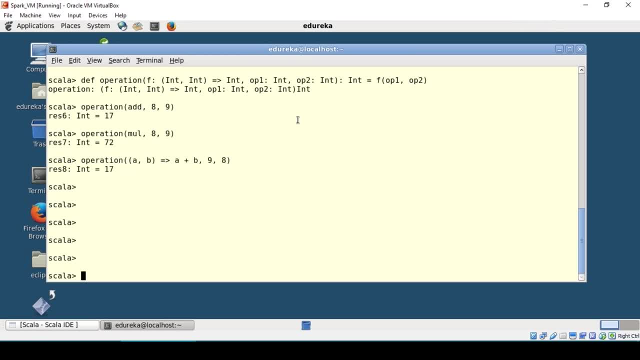 You know, in Spark. you know, instead of using this VM, I actually want to show it to you in a cluster. So let me see what I can do. I can actually show you some stuff in cluster and show you how stuff works. 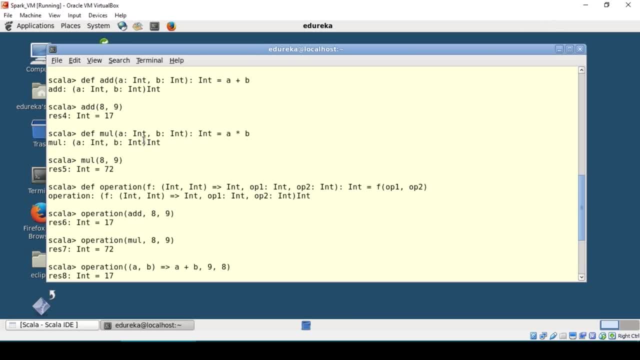 Okay. So now the thing is, you must have noticed one thing that you noticed: Add. you know, if I want to, I have to define an add function, I have to define a multiply function. It can actually become very boring, you know, to actually define this one line functions. 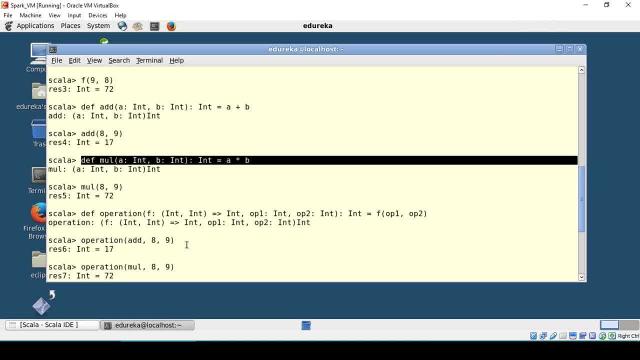 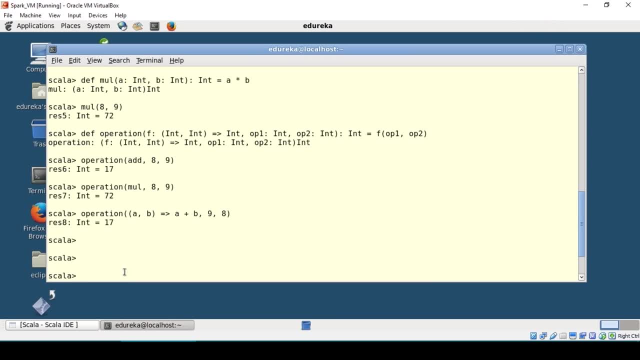 And then your source code, you know, will be littered with one line functions. So there's a concept called anonymous functions. Okay, Anonymous functions basically means that a function without a name. So what you can do is, you know, you can actually call operation and define the function. then and there, 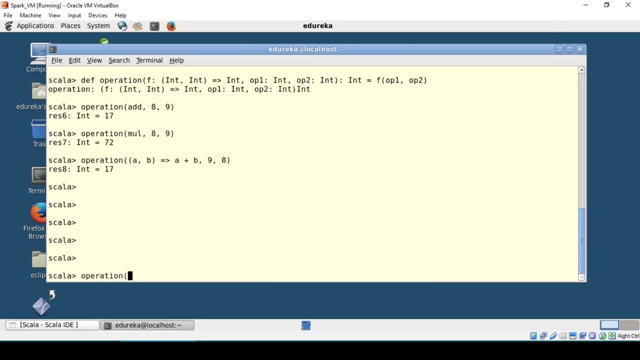 Okay. So what I can do is, when I call the operation, okay, I can then- and there you know- define the function. So I can say A and B, you know, and I can say that, you know, it's equal to A plus B. 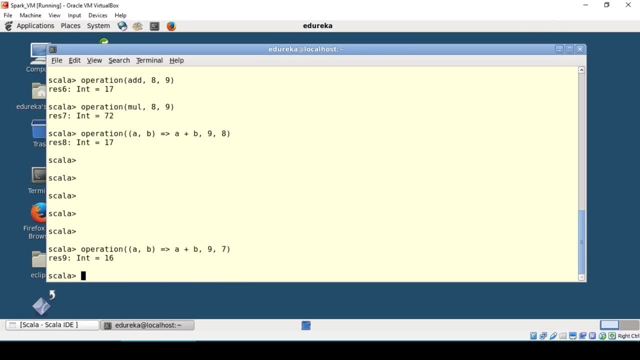 And then I can pass, you know, A and B, any value. Or similarly I can define an operation like A into B- Okay, It will be multiplied. And similarly I can do A divided by B. So that's also one. 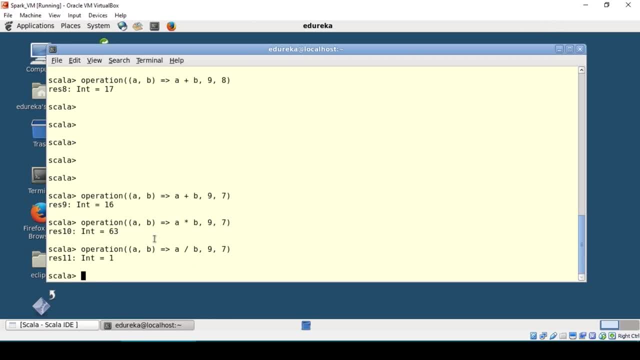 Okay, It does a you know modulus arithmetic here. So the thing is, here these are called anonymous functions. That means you know I didn't want to define the function outside because if you look at the multiplication implementation it's just a one line function. 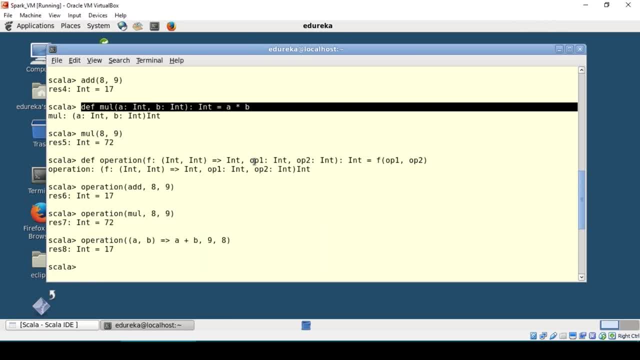 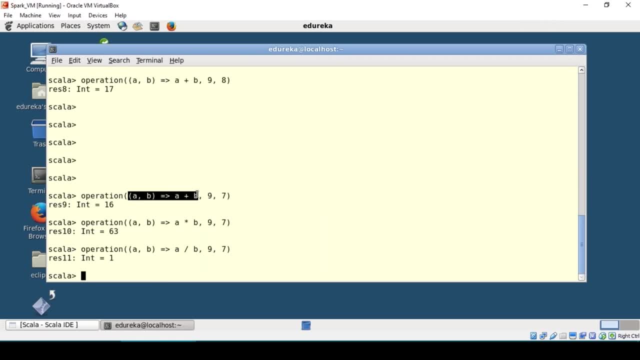 So I don't want to litter my source code. It's just one line functions everywhere. What I did was, you know, I just wrote anonymously one function. So this function here it's a definition itself. It's very similar to lambda expressions in Python. 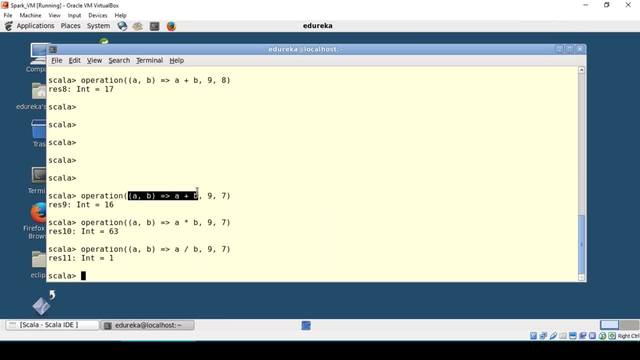 People who know Python will know this as lambda expressions. So it's just like that. Okay, So I define the two variables here A, B, and then I say A plus B. Okay, It can be any variable name, It's not A B. 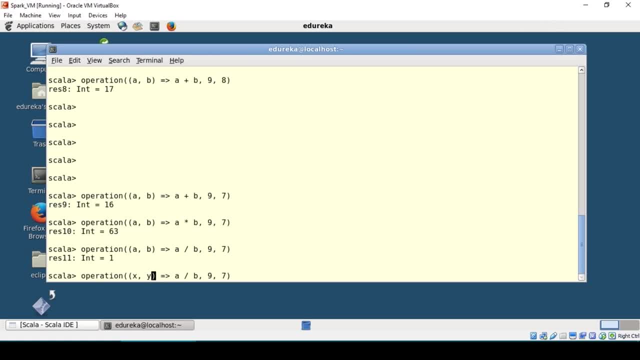 You can give X, Y also. You can name it after your- you know, your- pet dog or pet cat. It's no big deal, Any valid name will do. Okay, So it can be X plus Y. So basically what we're doing is we're defining the function right away. then and there, 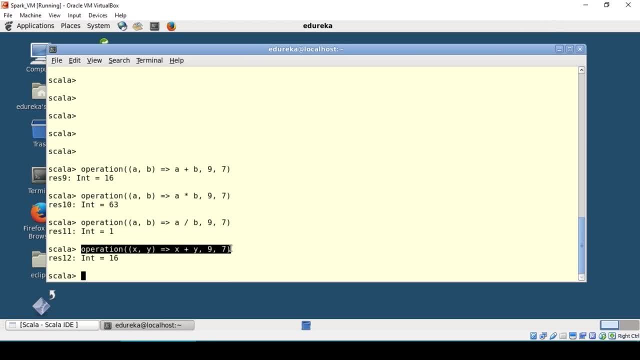 Okay, So that's basically the. these are called anonymous functions. Clear, all of you with this particular syntax. So you provide the parameters here, You don't have to provide the data type. Okay, So some of you may be wondering that you know where is the data type. 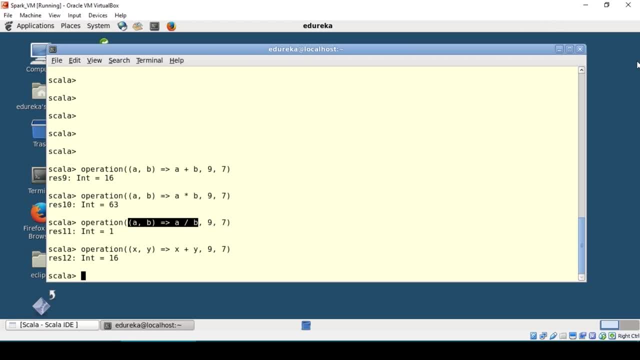 You don't have to provide the data type because the data type is automatically inferred from the parameters you're passing. But in case you want to provide the data type, you're free to do it. Okay, Nobody basically stops you. Okay, Ganesh is asking me: can we call anonymous functions in multiple places, or is it a single implementation? 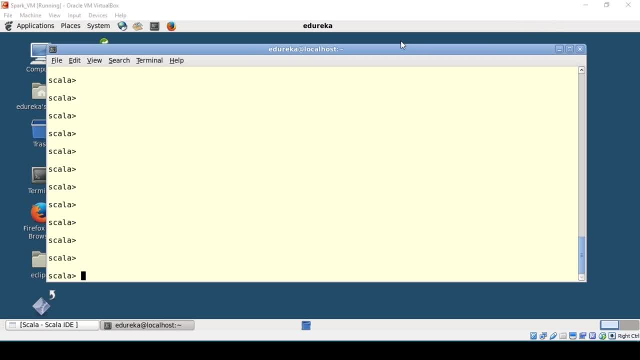 No, you can call it in multiple places. Ganesh, you know anonymous functions. wherever you know you are Anonymous function. the application is that you know when you you know when you pass a function as a parameter to another function. 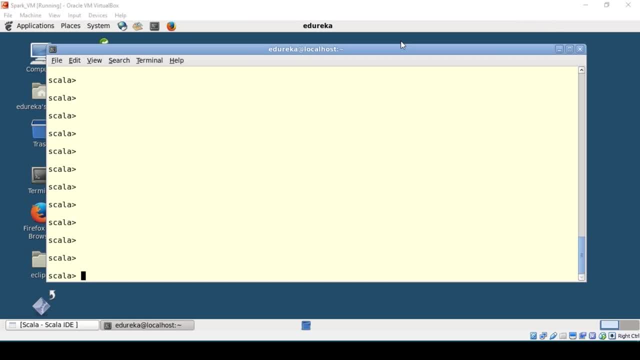 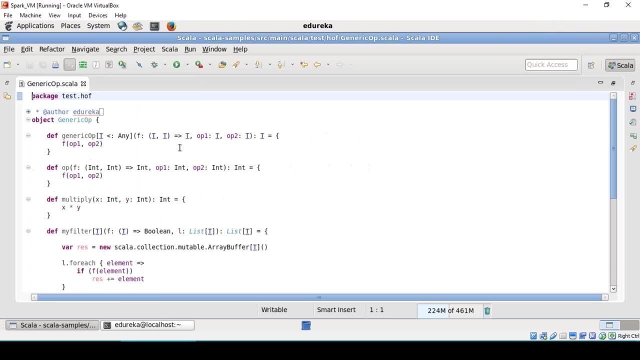 and if the function is very small, you can actually write an anonymous function. And let me show you some examples now in how we can do anonymous functions. So, firstly, you know, whatever that generic operation I did, you know, if you want to actually make it very generic form, 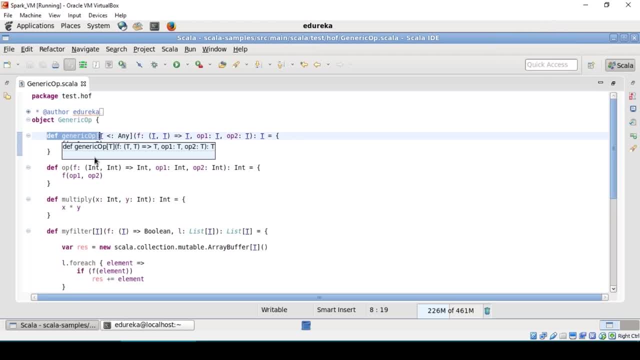 any data type. so actually you can define it like this: So you can write a generic operation. you know you can write it like this: a generic operation. Let me copy and paste it so that all of you are clear. So what you can do is: you know you can write the function generic ops. 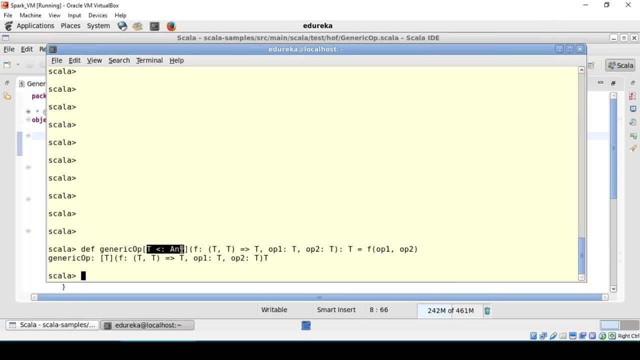 Okay, And you can say t. you can say that t should be a subclass of any, so that you don't pass any strings or nonsensical values. So it should be a subtype of any which basically is given by this sign. That means it should be a subclass of any. 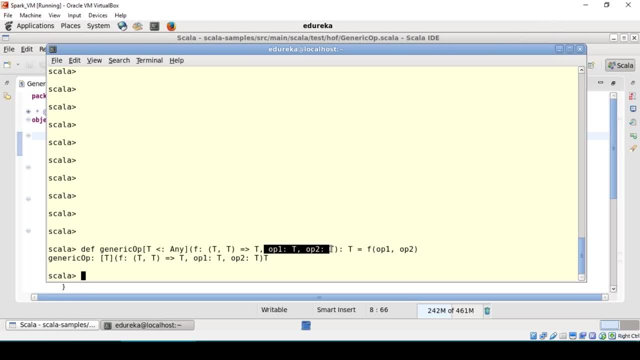 And then you say f, is you know of this signature and the operands out of this? So I just replaced the t with the float or the integer. Sorry, I just replaced the integers with t And the only extra thing I did was after the function name, in the square brackets, I wrote this: 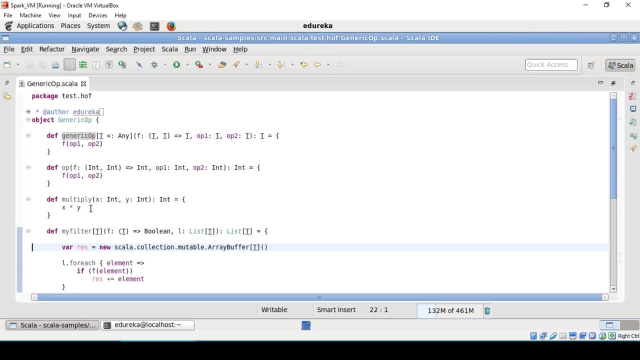 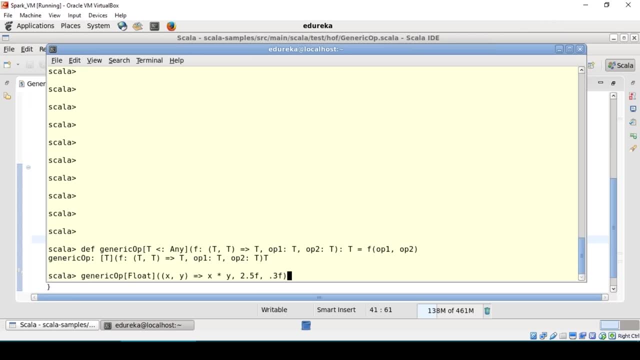 So now you can actually pass any stuff here. So if you want to call this, you can, you can, jolly well, you know, call it like this. So if you want to call it for float, so you can say generic ops, you can write float here. 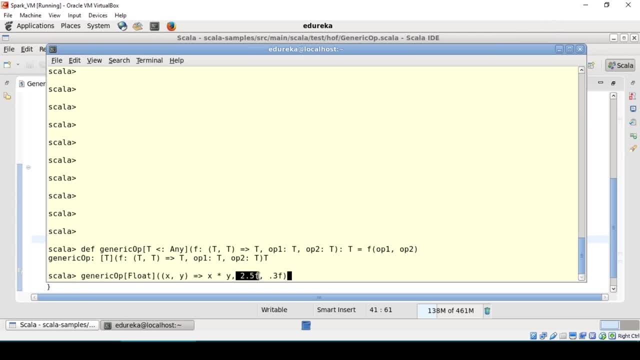 And then you can say x, y, It goes x into y, And then you pass 2.5, f and 3.. So this brings 0.75.. Okay, Similarly you can. you can try it for float. 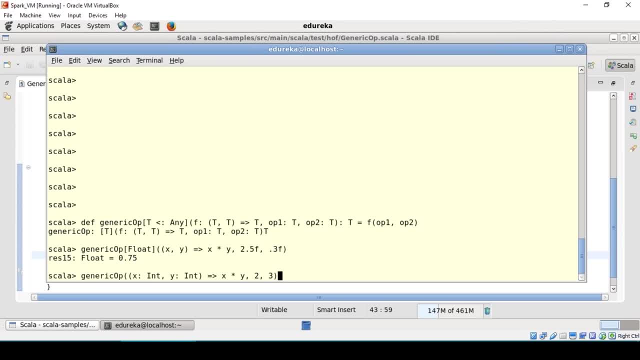 So we tried it for float. Now we can try it for integers, So we can just define the integer here, Okay? Vimla is asking: can the anonymous function have more than one line of code in the body? That's a very interesting question, you know. Vimla is asking. 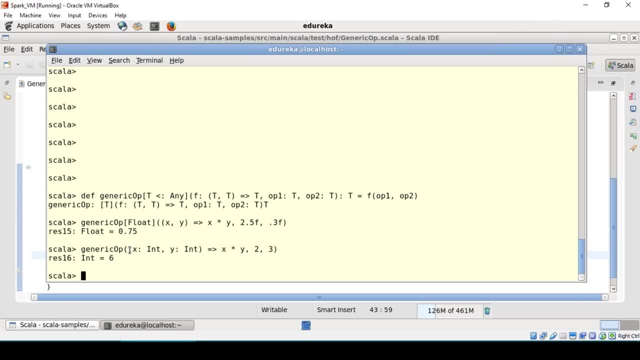 Vimla is asking that: can I have more than one line of code in? you know, in my anonymous function, The convention is, you know, just to keep it to one or two lines. Okay, So between two, three lines of code it's okay to have an anonymous function. 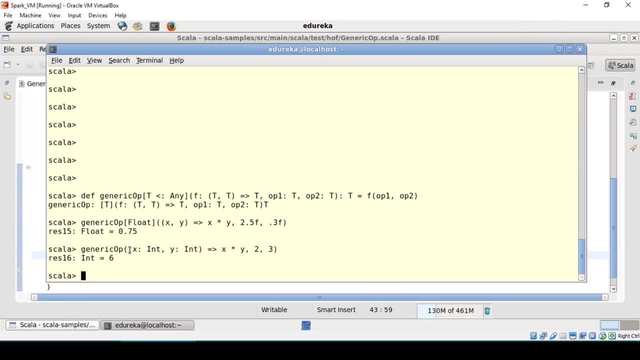 But if you're writing some 10,, 20 lines of code or more than that you know, then obviously don't write it as an anonymous function, because then it will your code will become extremely unreadable. So if it's between two, three lines, it's absolutely fine to write anonymous functions. 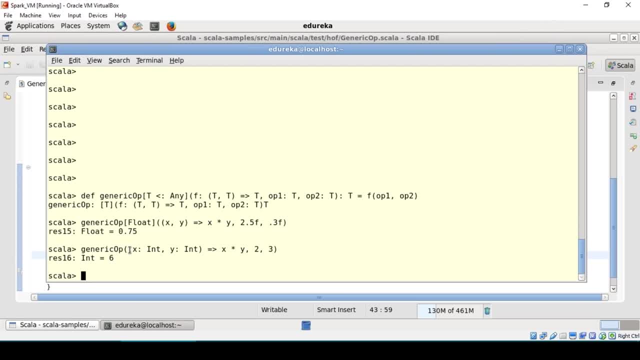 Okay, Okay. So Rafaela is asking me that: do they all have the same type or can I set op1 to different and op2 to different? Okay, Vimla, sorry, Rafaela. Rafaela is asking me that can I have? can I make different types? 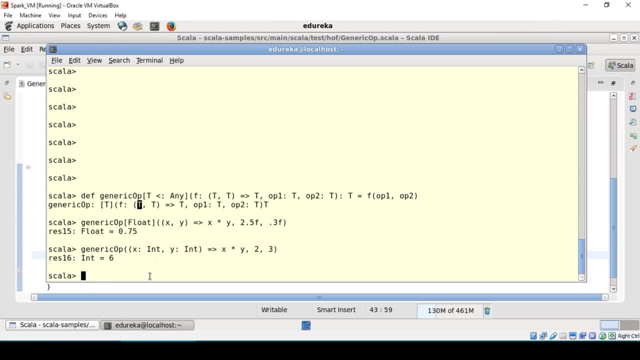 So can I have T of you know something and T1 of something? Absolutely, You can do that. Okay, So you can, you know, make multiple types also. You can make this T, you can make this of type U. 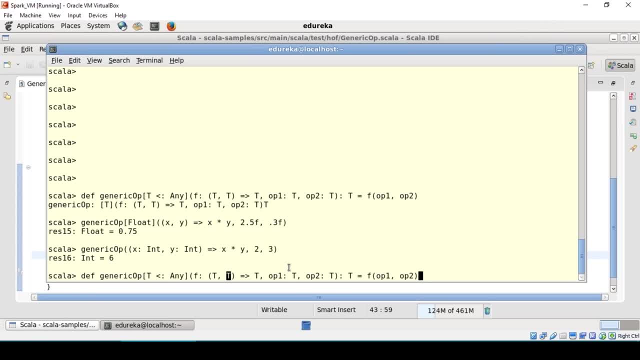 But the thing is that you know it should be addable, like the sense, in the sense that you know when you're adding a float to an int you have to cast, you know, an int to a float. 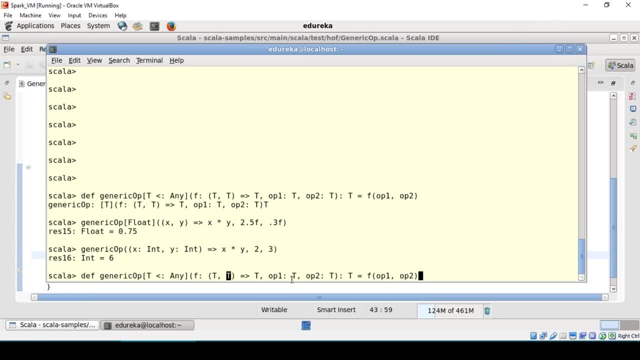 Okay, So internally that casting has to, you have to support that. Or when you're, you know, adding an integer to a double, you have to first upcast, you know, the double, the integer to a double, and then add it. 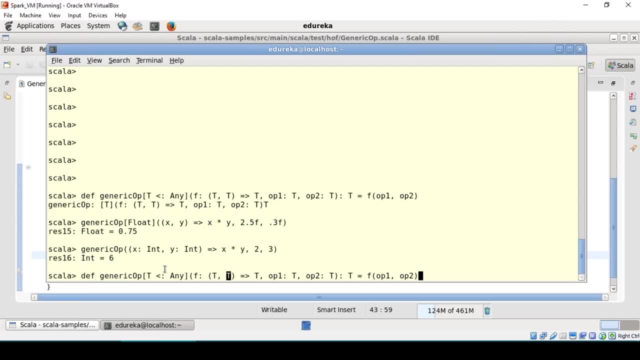 It becomes a little bit complicated in terms of the code, but you can do that. Okay So, but it's better to add you know same types. then then actually your code looks much neater. Otherwise you will end up, you know, having you know T, you know subclass of any and 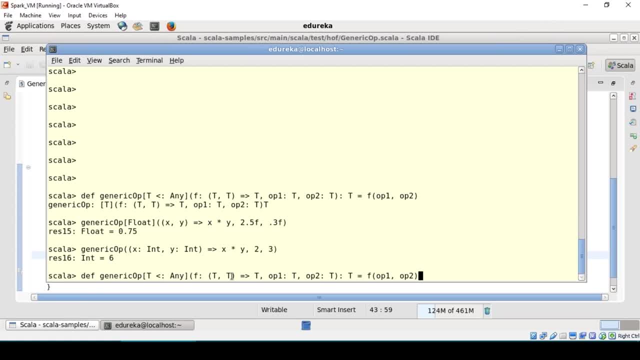 then you write another type, U, subclass of any, and then you write F, T and U, returning T, you know, and all these things you have to do. Yes, you're right, You know. Ganesh is telling me that you know, T, a subclass of any. you know it's redundant. 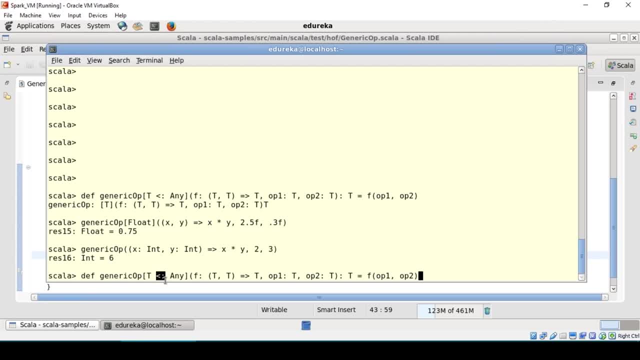 Obviously it's redundant, I know. I can show you that you know this particular operator. in case you want to subclass, you know this becomes very useful because any, any class in Scala you know, is derived from any. 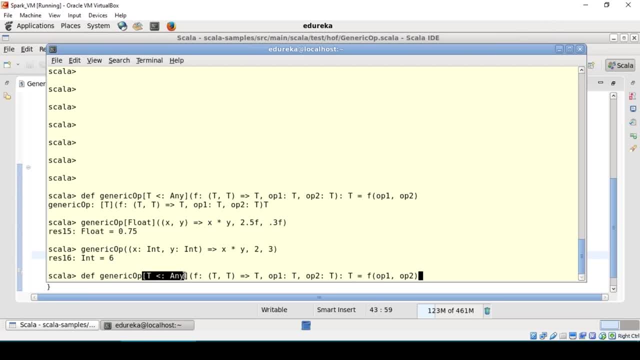 But say, for example: you know you are, you know you are trying to do a generic operation on a bunch of customers and you want this customer, or maybe a set of bank accounts, and you want to, you know this T to be only subclasses of accounts. 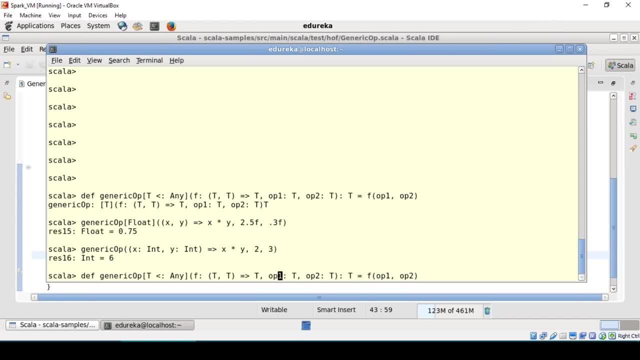 So then you can actually write something like this. you know, then it becomes, say, if you want T to be only subclass of accounts, so that people don't pass cat, dog, rats here, so you can do something like this: So only you know, subclasses of accounts will be taken. 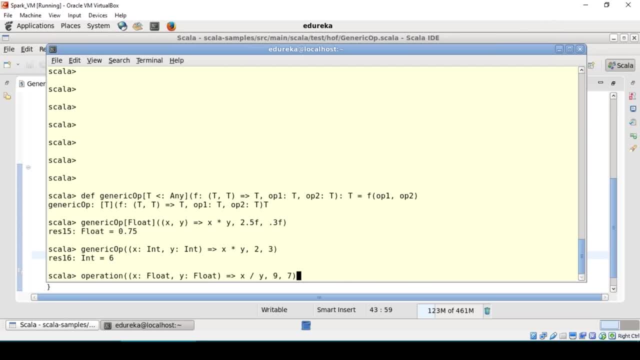 Okay. So this kind of thing Got it. Ganesh, Oh, okay, Good, Okay. So so that's about you know generic operations. I'm going to show you some more examples on on functions. So basically just to go back and review, and this is source code is there in my GitHub. 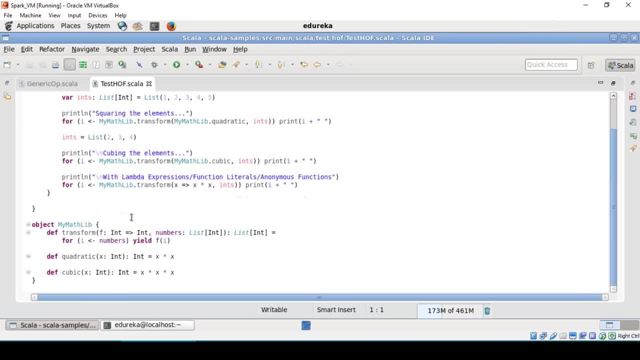 so you can download it and and have a look. There's another example. you know I can, I can give you, you know, when you typically want to do. you know transformations of: okay, no, I'll, I'll get. I'll do that, you know. 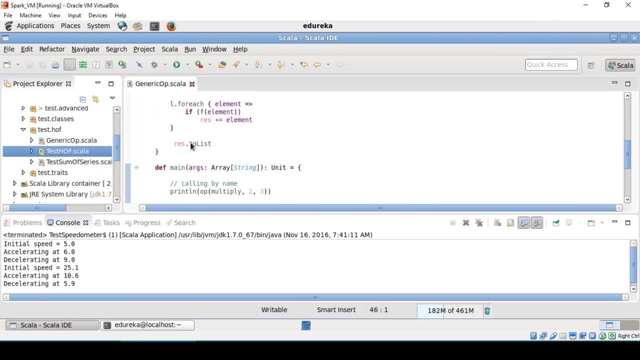 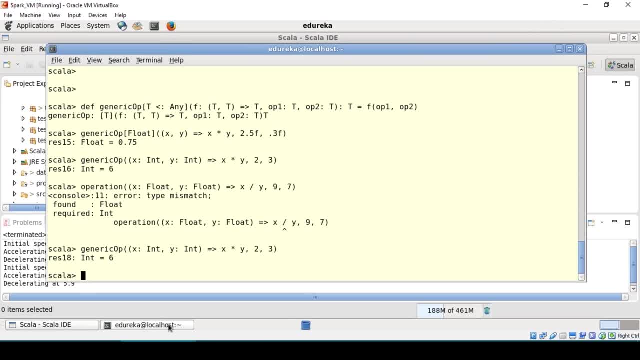 Okay, So that's about. you know how you do anonymous functions. So it's clear that Okay, Praveen is asking me: does it have any name calling function? you know function definition. Sorry, Praveen, I did not understand your question. 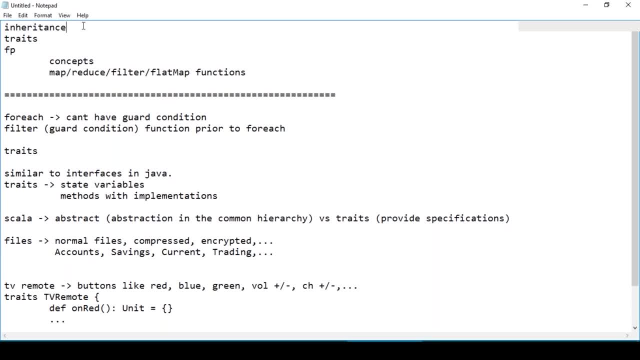 Maybe if you can rephrase, Okay, So let's quickly review. you know we have done inheritance, so that's basically done. today We did traits, that's finished. a function programming concepts. You know I explained to you what first-class citizens are. 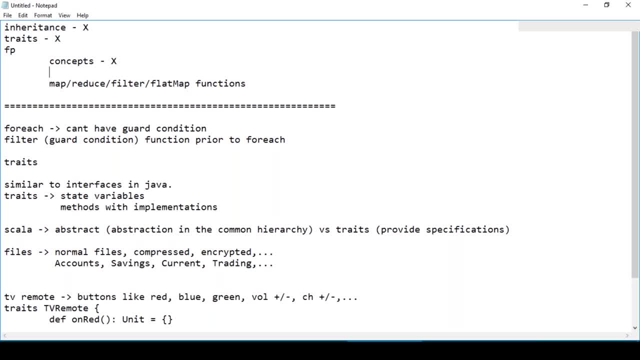 what higher-order functions are. I gave you higher-order functions examples. I explained to you anonymous functions and their uses, so you know when to use anonymous functions and what are their uses. okay, sorry. So now what we're gonna do is we're gonna look. 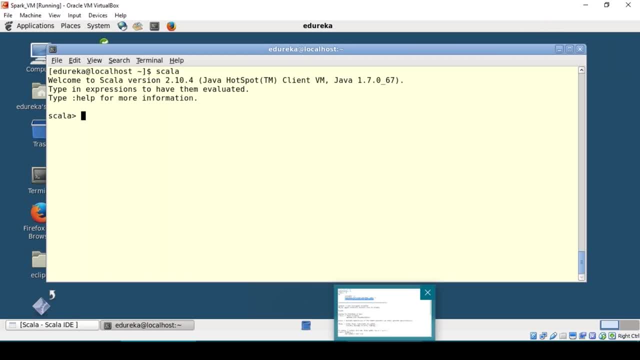 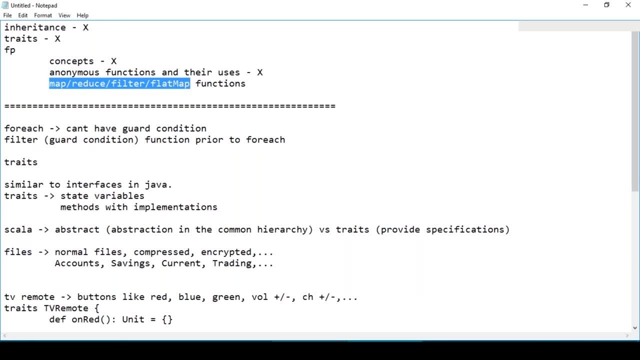 into some more examples of application of higher-order functions and anonymous functions. okay, So we're gonna look into four important functions: map, reduce, filter and flat map. okay, So what are they? So let's take a list. you know L. 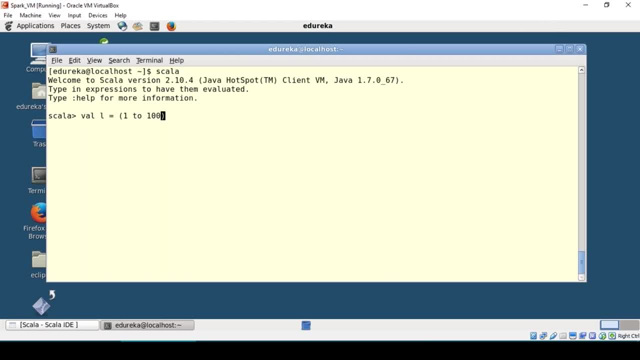 and let's take a number from one to 100, or maybe let's keep it simple one to 20, and I convert to list. okay, So now I have this numbers one to 20 as a list. Now the first function which I'm gonna teach you. 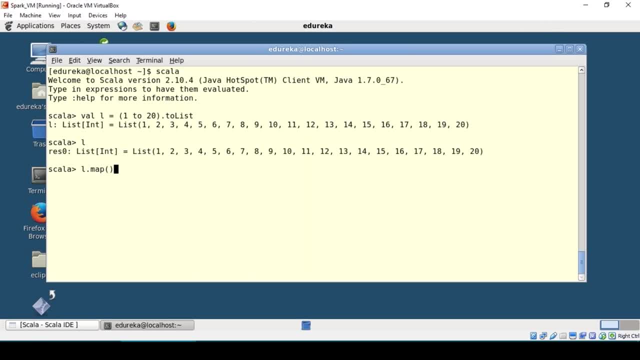 is something called a map, okay, So map what it does is it basically applies. so the map function basically as an argument. takes another function, Okay, and this function, basically what it does is it does a transformation on each and every element of the list. 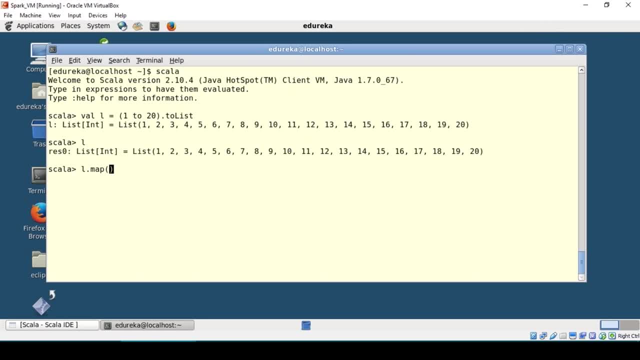 So say for example, I pass a function here, say for example n, and I say that n into two. So here what happens is basically: it means that you know, this is a function definition, n into two. So that means every element, okay. 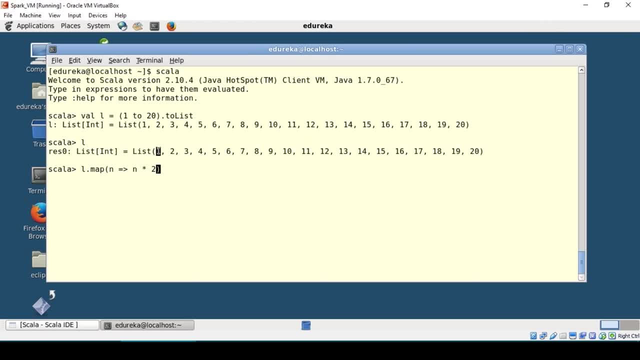 every element of the list will be multiplied by two, So that means every element will be passed through this function: n into two, So n will become one, one into two, then again n will become two, two into two, then n will become three, and then three into two. 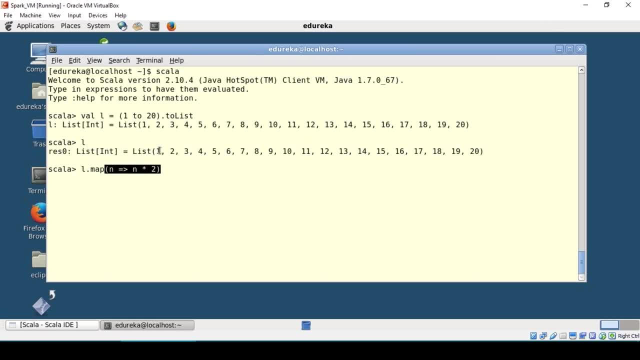 like that. okay, So this particular function definition will be applied to each and every element. Clear all of you what this is? And if I run this, you'll see that all the elements have been multiplied by two. Is this clear to all of you? 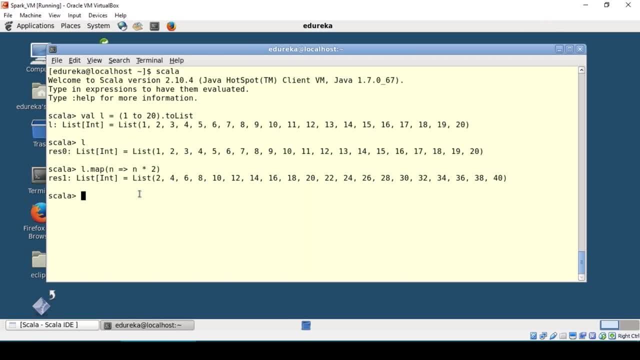 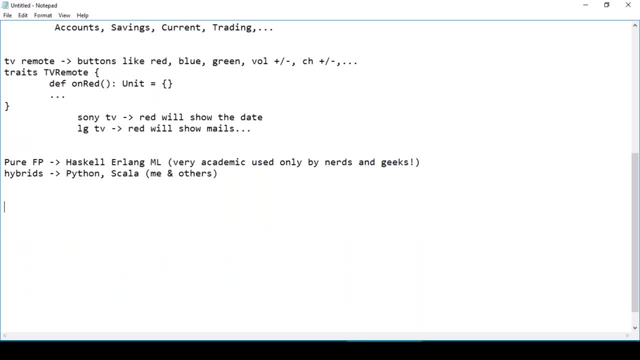 And you know there's a very interesting question which Vimala asked us, that: is this map anything to do with map? you know the plus map, okay, We learned that. you know, yesterday we learned class map okay, which is nothing but a hash table. 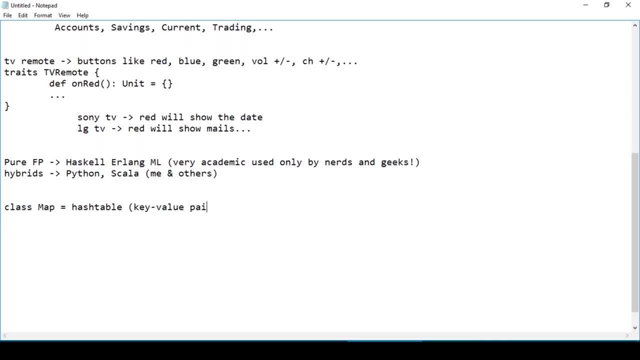 So it's a hash table, okay, of key value pairs. Now, this map function, you know, has nothing to do with the map class. okay, Just remember this please. So it has nothing to do with this. No, Srinivasa, you cannot do that. 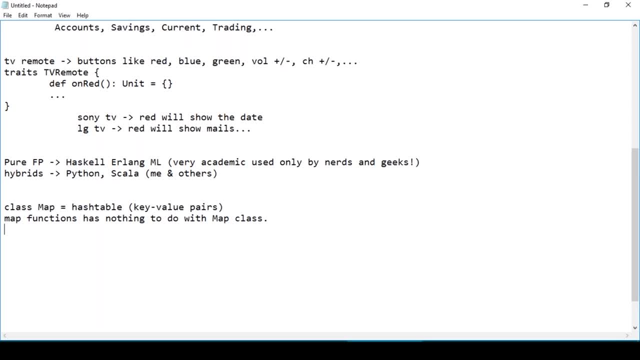 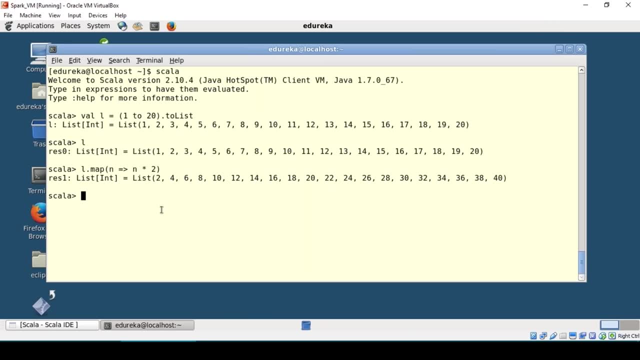 It doesn't make sense, okay. So what you're saying, Srinivasa? that's the wrong syntax. You cannot do this, Okay. so, yes, you're right, Rao, You can use this to provide transformations to the map. 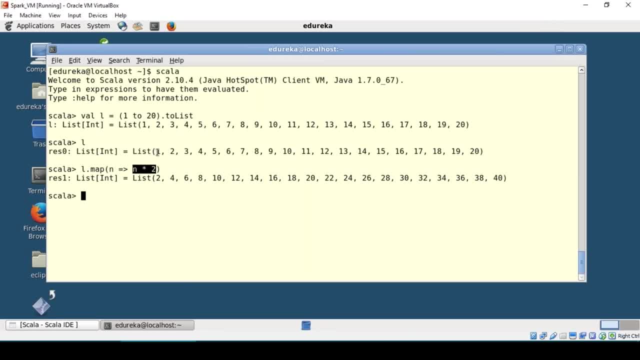 So if you want to multiply this map- you know each and every element by two, you can do this okay. So, similarly, if you want to say, for example, you have a string you know like test, So you can say strmap and you can say each character. 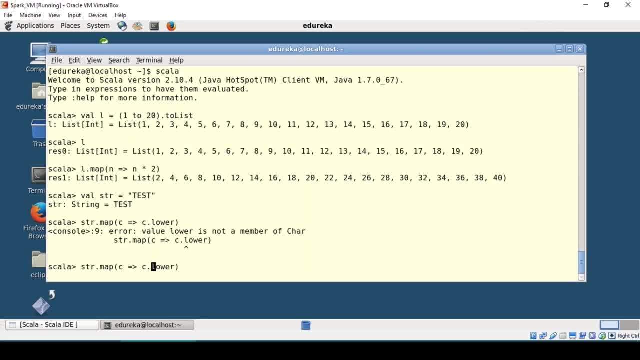 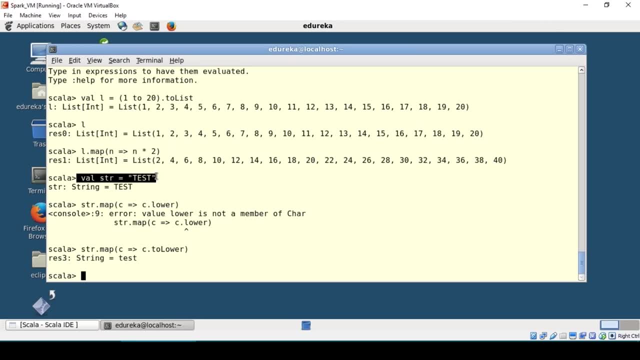 you know, characterlower. Sorry, what was the function? I think it was too lower or I forgot the name of the function. Yeah, too lower. So what it does is, you know, I have a function called test, sorry, a string called test. you know, all in caps. 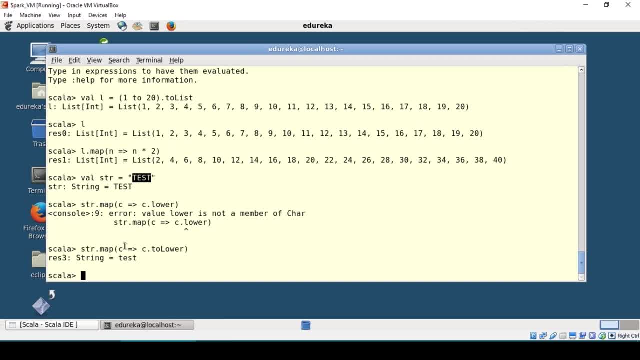 So now what I do is: you know, I want to convert this whole test to a smaller case. So what I can do is: you know, I can call each character, I can pass each character. I told you that string is like an iterator. 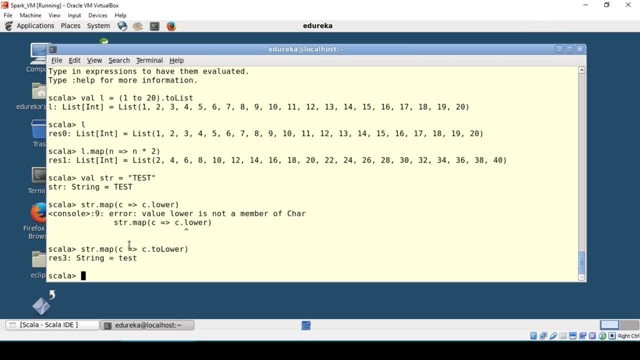 So the map can be applied to any iterators, which is where every element is iterable. So here what happens is each character in the string is passed, you know is called with the function too lower, and then each character is reduced to a lower case, clear. 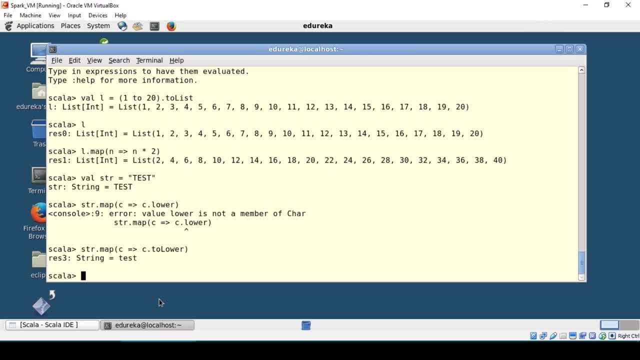 So that's applications of map. Now the thing is, you know Scala. one reason why Scala becomes a little bit difficult to master is because you know Scala has a variety of syntax. So this, you know this thing which I wrote here, 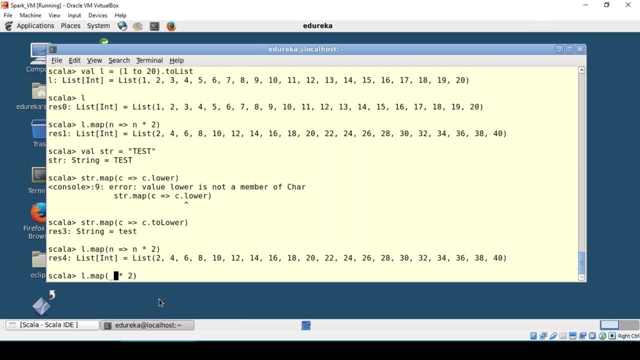 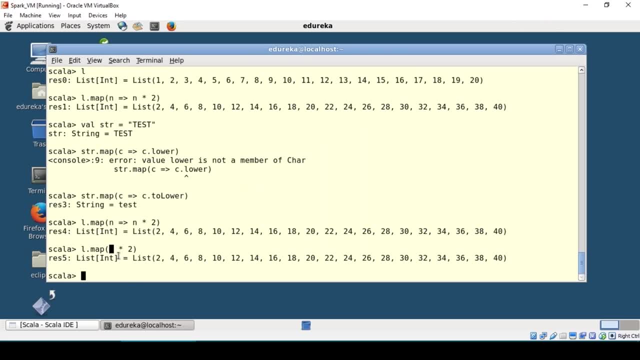 this lmap. this can also be written like this: okay, So it can also be written like this: This is called a wildcard, okay, in Scala, which basically means that you know this underscore. it's like a wildcard, so that means every element. 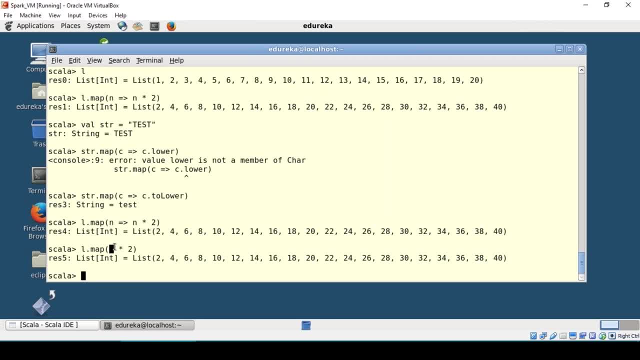 of the list will be substituted here and will be multiplied by two. So this is also a function definition in the wildcard form. Okay, so you give an underscore here, which means that every element of the iterator of the list is going to be substituted here and multiplied by two. 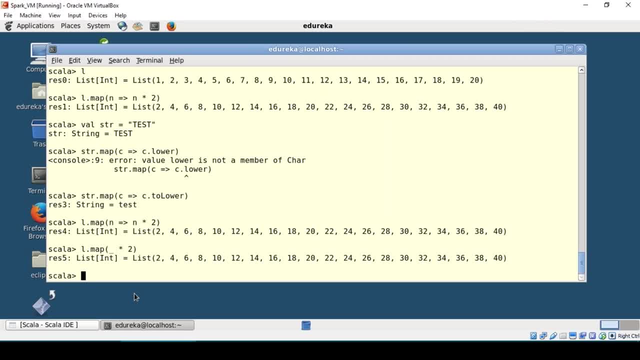 Okay, so you can use either this syntax or this syntax. Both are fine, whichever is comfortable, And both are functions okay, So don't think that this is something else. This and this function is exactly the same. So the function definition here and the function definition. 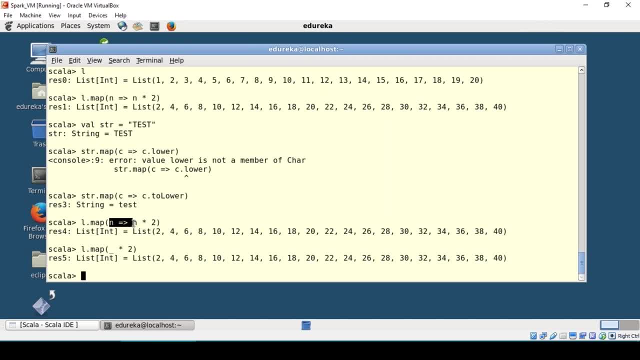 what I've written is exactly the same Here. instead of n, this function here like this: you just write an underscore, clear. So that's a map function. So map is basically. you know, if you want to transform an element. 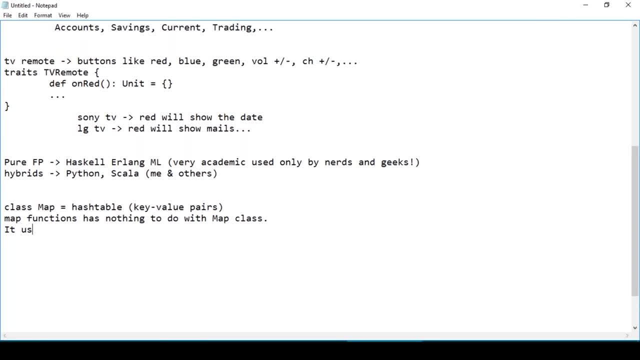 so let's write it down. So map function. nothing to do with the map class. Okay, it is used for transforming individual elements in an iterable collection. clear All of you what a map is. I gave you two examples, one with a number. 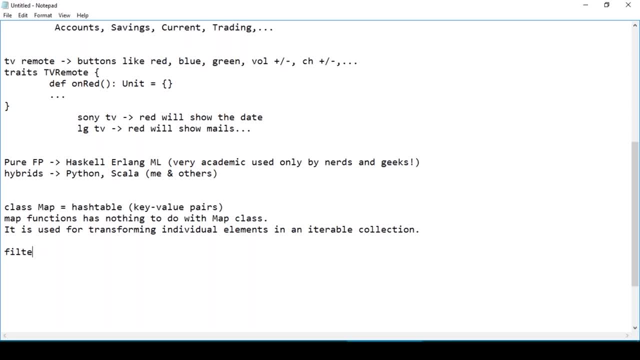 and another with a string, Okay, so now we are going to learn the filter function. So filter is again, you know, it's just to skim out whatever you want, okay, And the filter function, you know, basically takes a Boolean predicate. 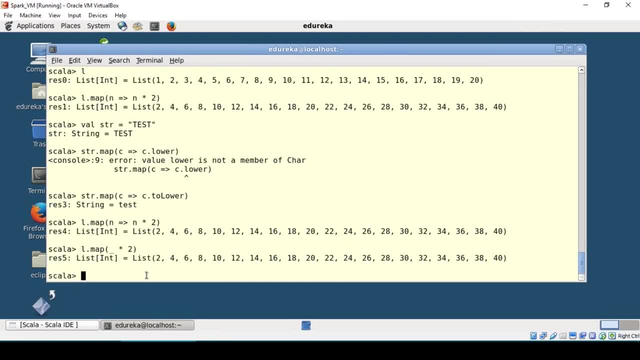 So what happens here? so let's understand this with an example. So here you know, I have this original list, And what if I want only the odd numbers from the list? Okay, I only want the odd numbers from the list. 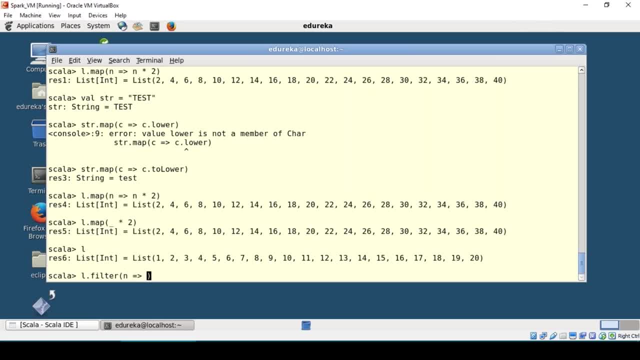 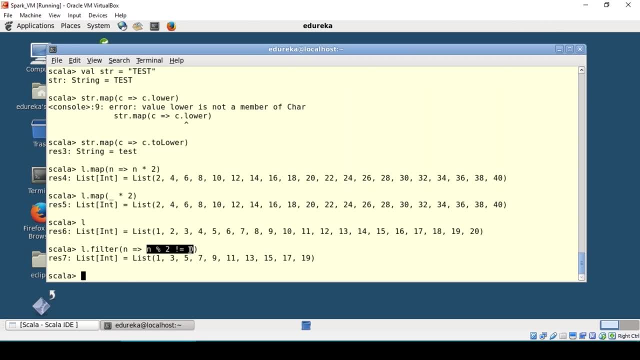 So what I'll do is I'll write a filter where I will say: you know, I'll define a function where n in a module of two not equals to zero. So I defined a function here where basically it's a Boolean predicate that takes. 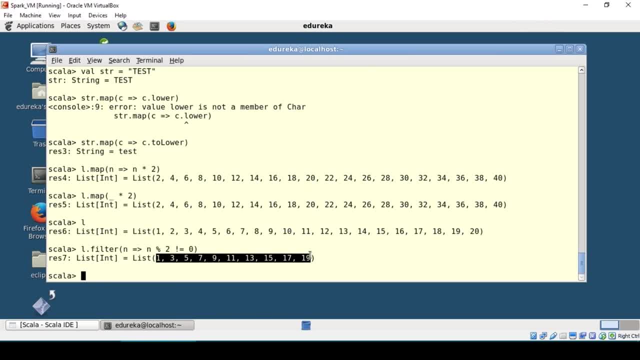 that n module of two not equal to zero. So then it basically gives me all the odd numbers. Okay, and you can write it like this also as a wildcard form. Both are absolutely valid, So this will also give me the same thing. 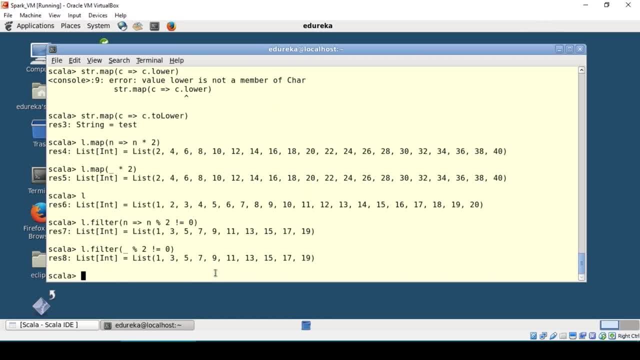 So filtration, remember, filter function you always use when you want to, you know, filter out something from the list. Yes, you're right, Ganesh, It's only used for collections, for traversable collections, And the expression should always have a Boolean. 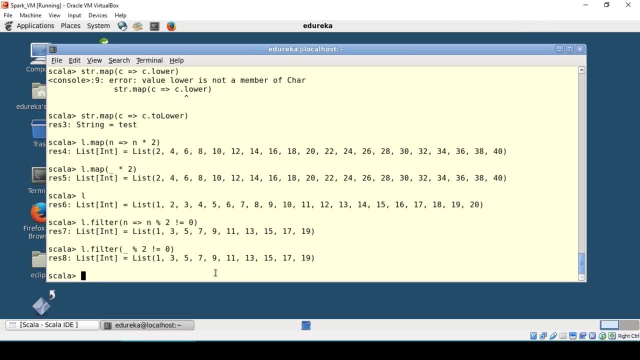 The return should be Boolean. Yes, right, Yes, Rao, you're right. Whatever you pass in the filter function, the return type should be Boolean. So that means the function here, obviously the return type is Boolean, right? So say for example: if you write: 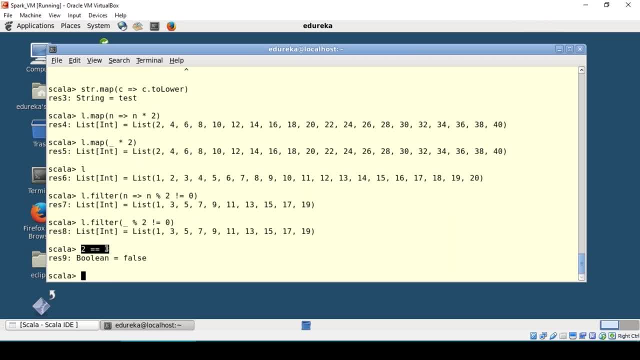 whether two equals two equals to three, you know there's a Boolean expression and the return is false. So, similarly, whatever function you define here, you know it should be a Boolean, The return should be Boolean. So that means it should devalue it to a Boolean value. 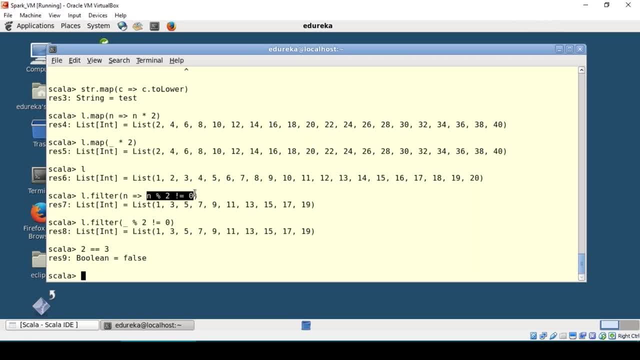 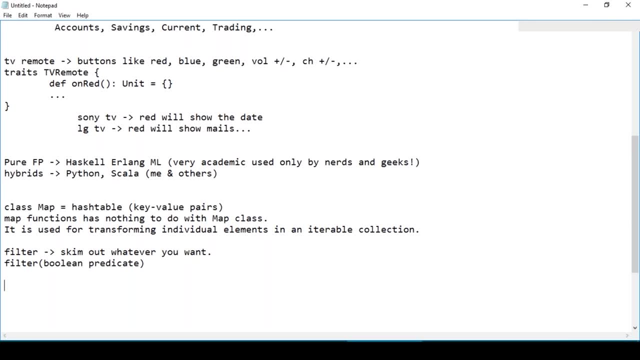 I'll come to that. Erwin Erwin, I'll come to your questions. okay, So that's you know, the filter. Now let me go to reduce function. okay, So the reduce function. what reduce function does is: 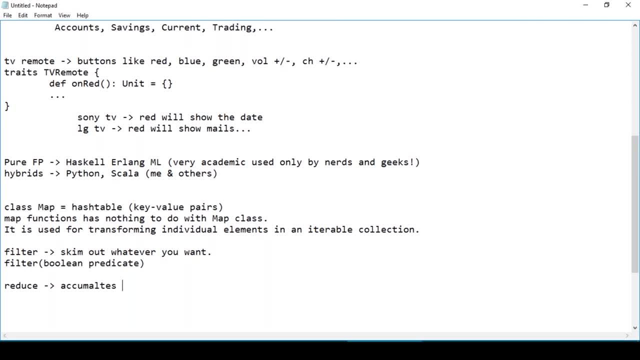 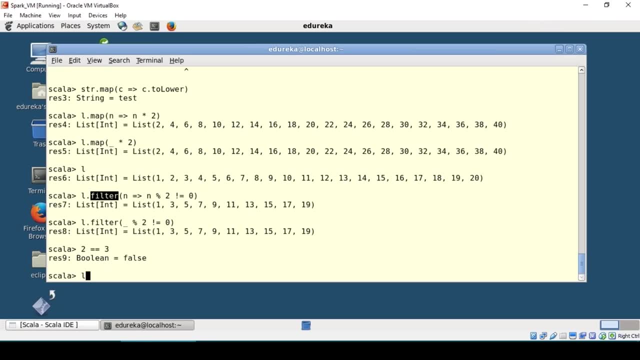 you know the reduce, basically you know, accumulates the value of the collection, So it's like finding the sum. Okay, so you have this list here, You have this list. So if you do lreduce and you write it like this: 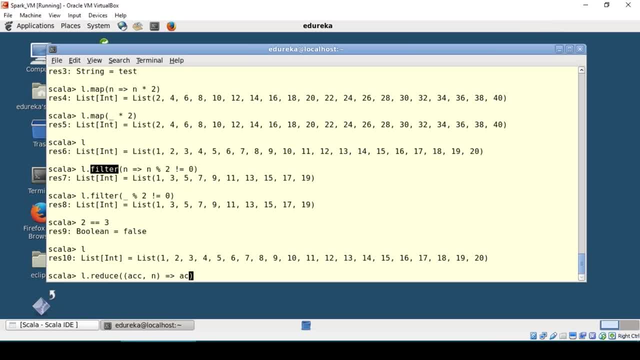 So this is the accumulator and this is the element, and you write it like accumulator plus element. So this basically gives the sum of the integers from one to 20.. So that's exactly 210, okay, So here accumulator is basically the counter variable. 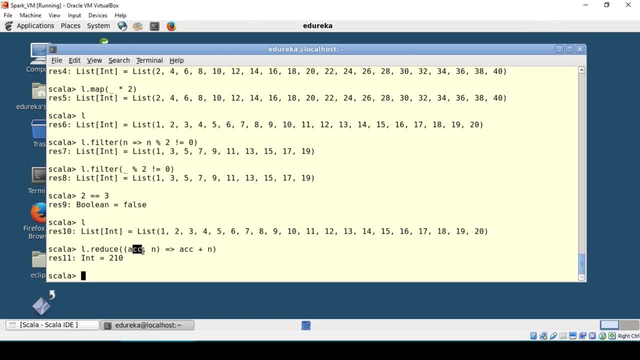 So it's one plus two, three. Three is stored here, then three plus three. six. Six is stored in ACC, then six plus four, 10.. 10 is stored in ACC like that. Okay, so it keeps going. 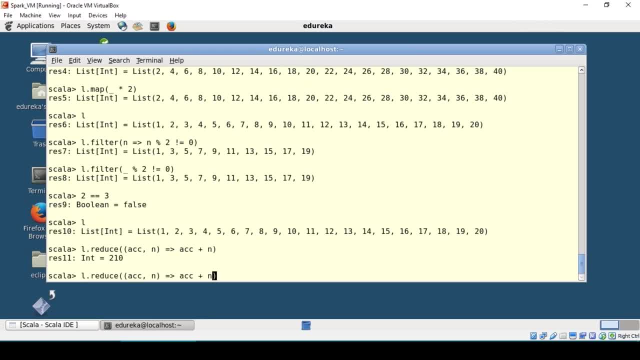 Clear, all of you. So that's the reduce function, and the reduce can be also written using the wildcard syntax which I've written before, you must be aware. So you can write it like this also. Absolutely fine, okay, Okay here. Rao is asking me that how ACC and n? you know? 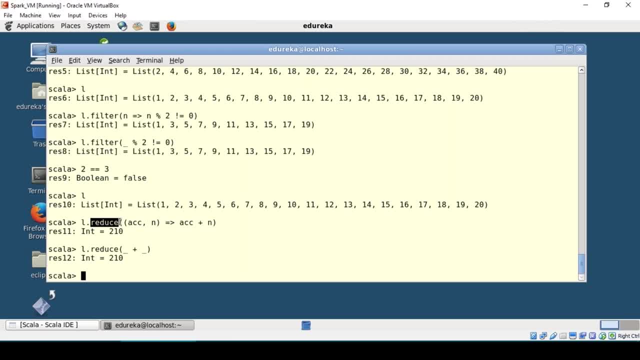 the default values. what happens is, if you look at the source code of reduce function Rao, you will see that you know when you're doing addition. basically, ACC is initialized to one because one is the identity- sorry, is initialized to zero. 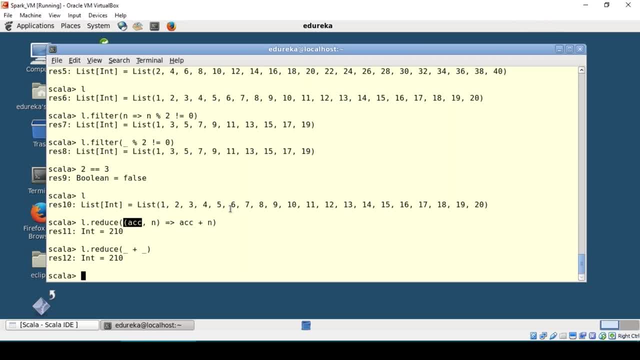 because zero is the identity for addition. and then you know, it basically goes through each and every element of the collection and keeps accumulating. that in ACC, okay. And similarly, when you're multiplying, ACC is initialized to one because identity in multiplication is one and it keeps on, you know. 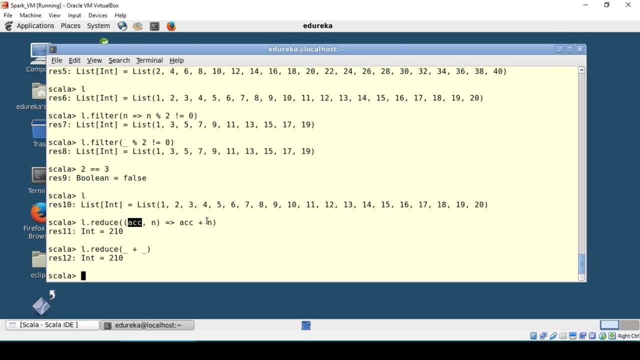 accumulating the multiplication values. okay, So that's how it gets the. it's basically based on the operation. it gets the initial value. okay. So if you look at the source code, you will see that you know the ACC is usually initialized. 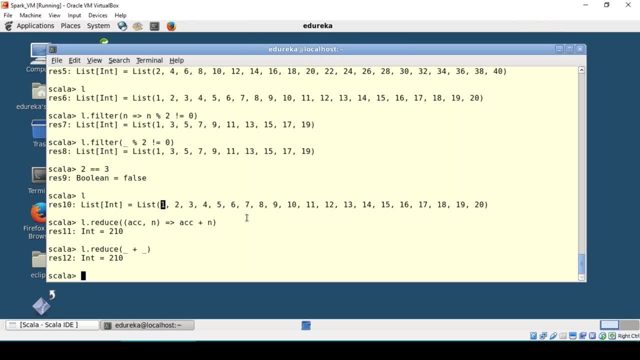 to the first element of the collection and that's how it keeps on doing the operation. okay, So if you, I don't want to open the source code. it's a little bit complicated, but in case you're interested, you can see that. you know the ACC will be initialized. 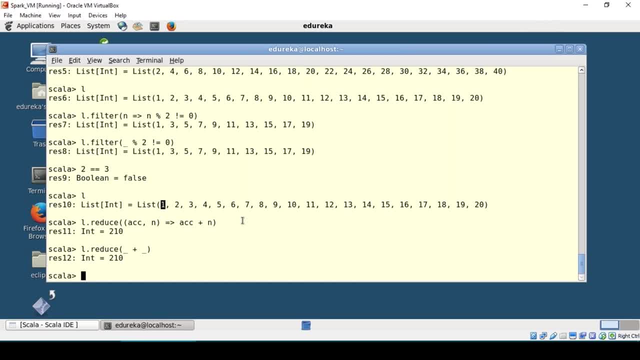 to the first element and then the counter will start. okay, Okay, Ganesh is asking me: will that be used for Hadoop MapReduce functions? No, this has nothing to do with Hadoop MapReduce, It's just that they share the names. 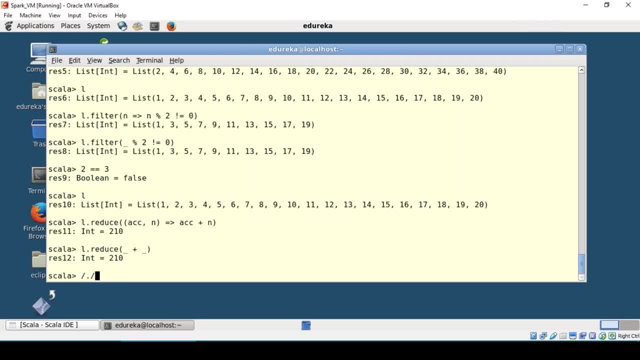 Okay, good, so these are the three functions we learned. Now, let's you know. see, one requirement: If I give you the requirement that, okay, we have this list. L, okay, What I want from you is that you know. 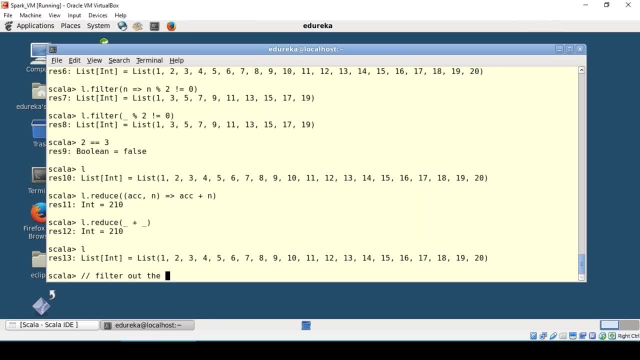 in a skim out or in a filter out the odd numbers, okay, Then square them and find the sum. So how am I going to do it? So I'm saying that you know, filter out only the odd numbers. then, whatever you've filtered out, 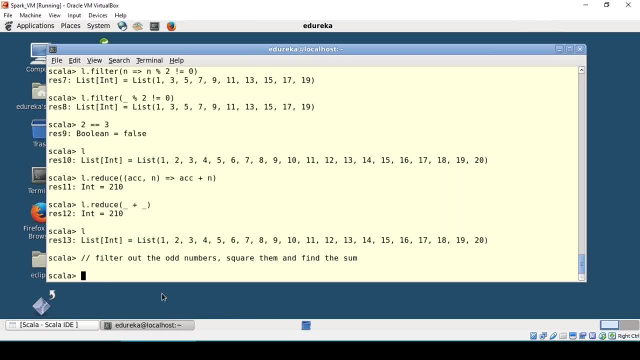 the odd numbers, square them And then find the sum. So how will you do this? So you will say Lfilter, and then you're going to say, you know, filter out only the odd numbers. So what I'm going to do is N modulo two not equals to zero. 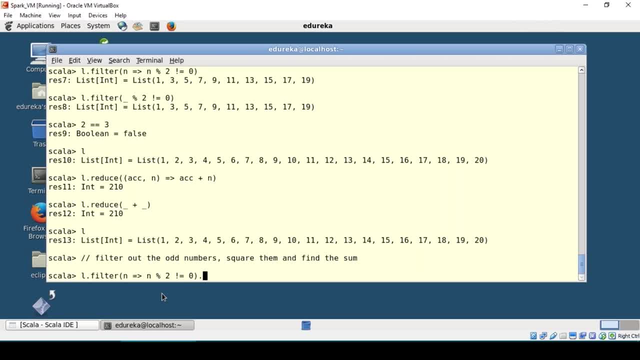 Okay, so I do that, So I filter out all the odd numbers, Then I'm going to square them, So I pass it through a mapping function, N to the power two, And then what I do is then I'm going to find the sum. 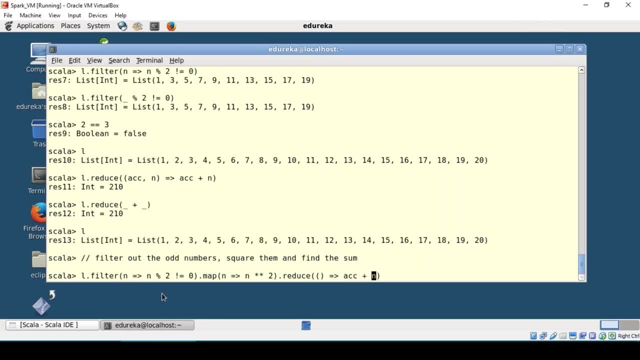 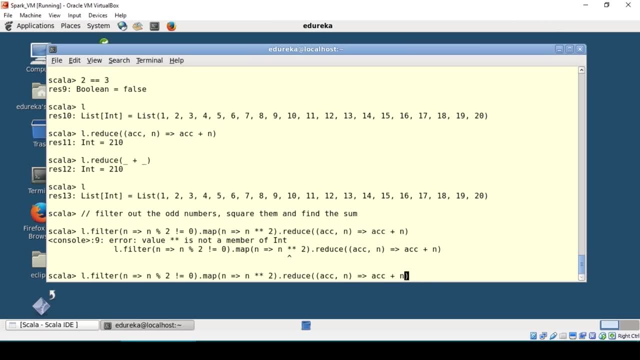 So I reduce them And I reduce it like this: Okay, oh sorry, this is a Python operator, So I have to use power power function. So you can use the power function N two And this will actually give you the answer. 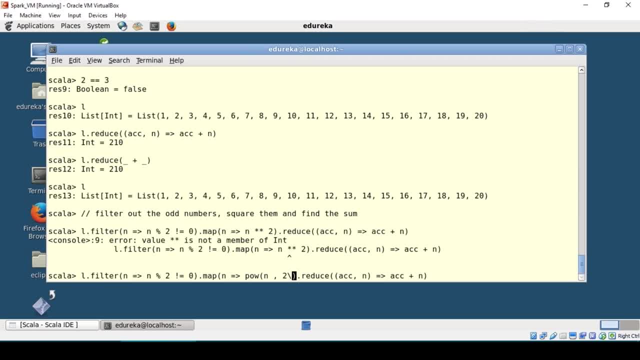 Just a minute. let's keep it simple. Can you all see my screen? Okay? so this is what I'm doing. So I'm going to filter out all the odd numbers, Then I'm squaring the numbers And then what I'm doing is I'm finding the sum. 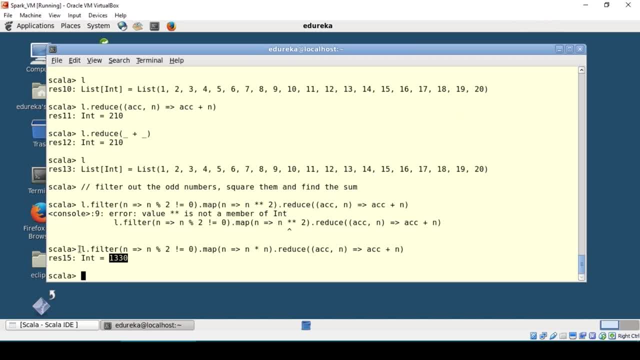 So if you do this, this is the answer which you get And you see, this is called chaining. You know this is called function chaining And you see that. you know how nicely I can get the stuff. You can also use a wildcard. 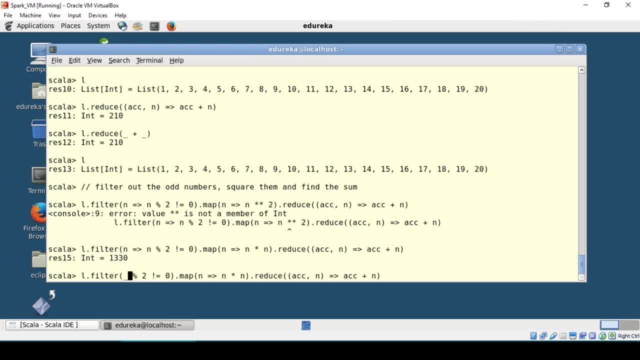 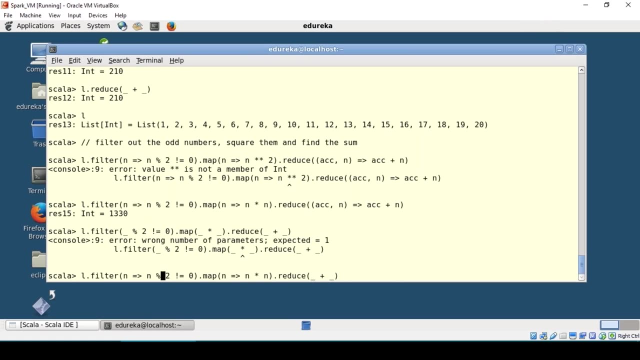 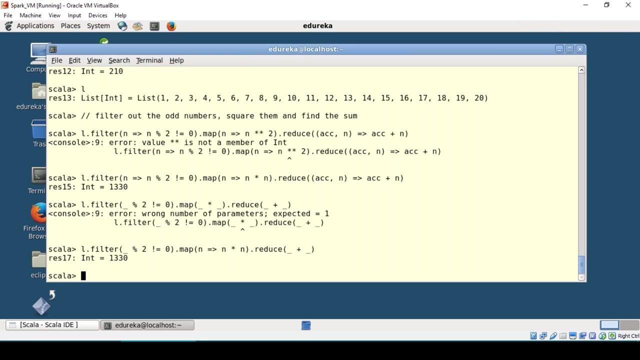 You know you can use the wildcard syntax to do this as well, So it's based on your convenience. you know how convenient you are in doing this. Oh, sorry. Okay, Ravi's asking me: in projects do we use the wildcard syntax? 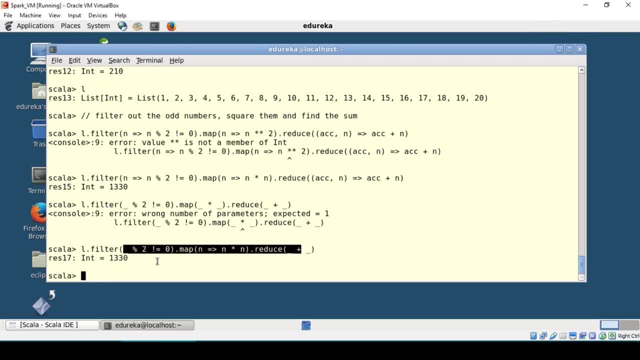 No, it basically depends on your preference purely. You know and check the organization where you're working. What is the syntax they follow, Because in some companies, you know, they strictly mandate this kind of a syntax, Whereas in some other companies they are okay with wildcard. 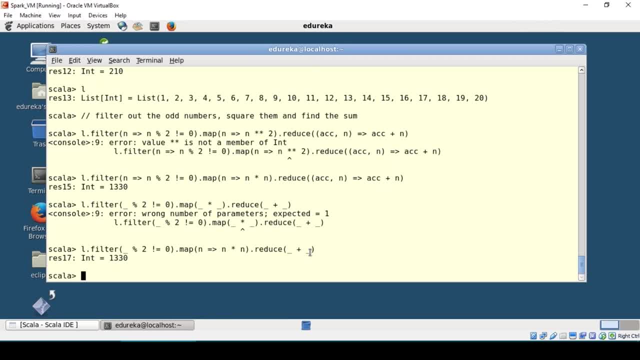 So just check what is the coding convention there. Both are equally okay. So, and I've seen most of the places where I've seen most of the places wildcard is used, There is no problem at all. But you have to check, you know, with your project. 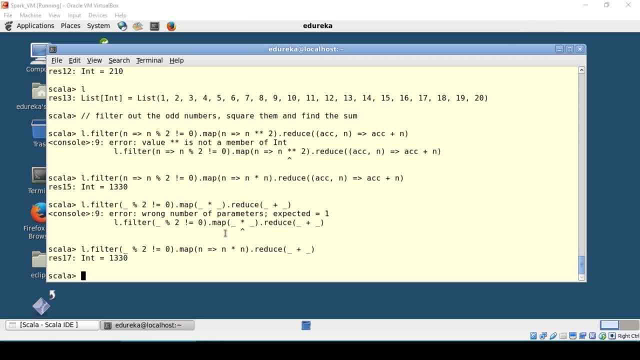 what they're comfortable with. okay And no, I got the above. okay, Venkat is asking me why did I get the above error? Because obviously you know, I'm multiplying a wildcard with a wildcard with itself doesn't make sense. 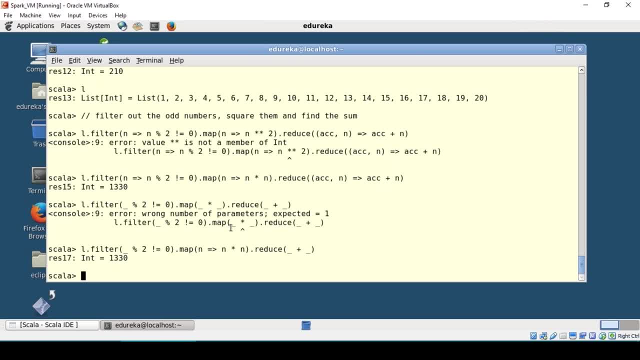 So there, you know I can't use a wildcard, I have to use a proper function definition. okay, So because the compiler gets confused, that you know I can't use a wildcard, What are these two wildcards here? okay, 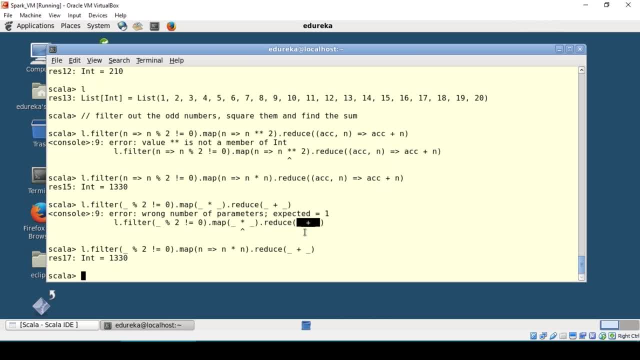 But this is not the problem with the reduce function, because in the reduce it knows very well It is just folding the collection. But here you know, in the map a confusion. It's the way the map is implemented. Clear Venkat. 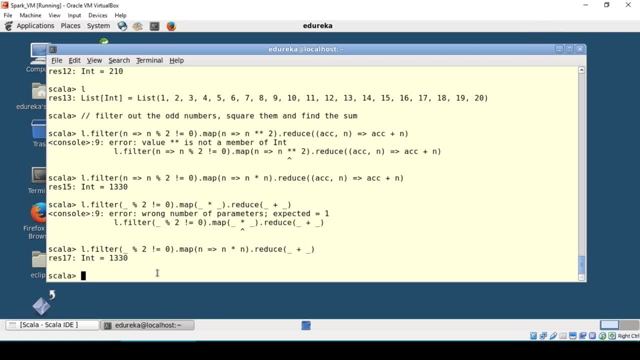 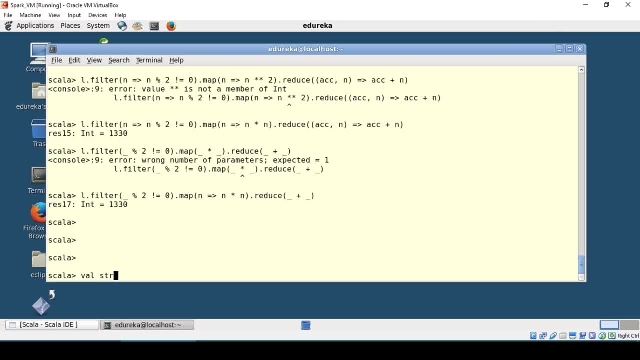 Okay, so that's about the map reduce and the filter. Yeah, you're right, Venkat Reduce has the functionality to understand which map doesn't have. So now let's do some more fun with things you know. Let's have a nice day, okay. 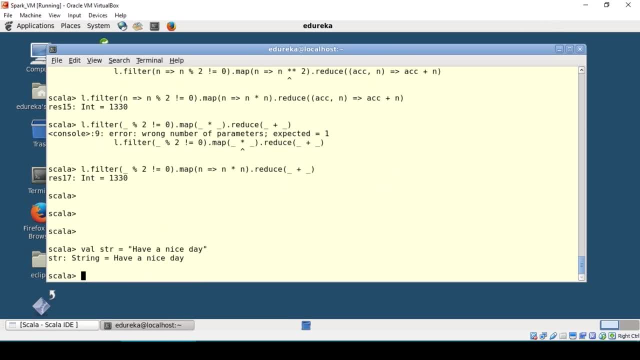 So this is the string I have. Let's do a word count, okay, of this. So let's do a word count. Shall we do a word count of this? Okay, so let's find out, you know to do a word count for this particular. 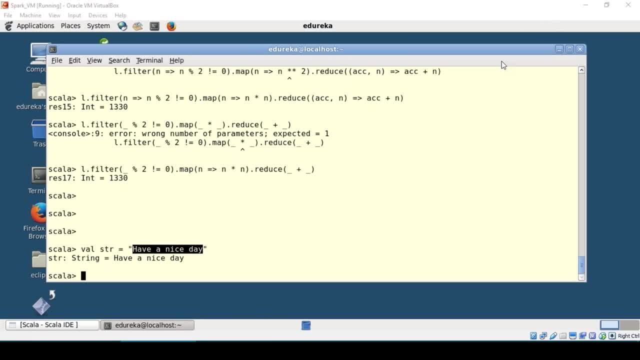 So here we have a string and I would like to do a word count, for you know, just count the number of words this particular string has. So would you like to do this? Do you want me to show it to you how this is done? 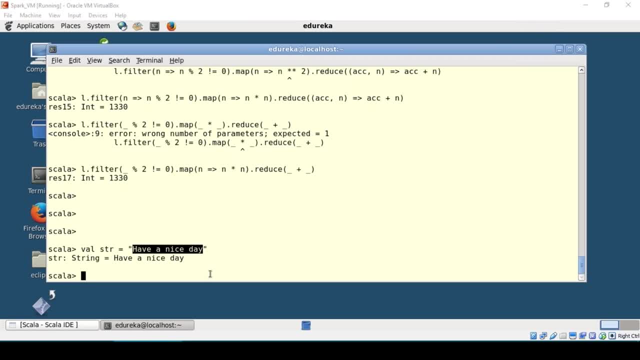 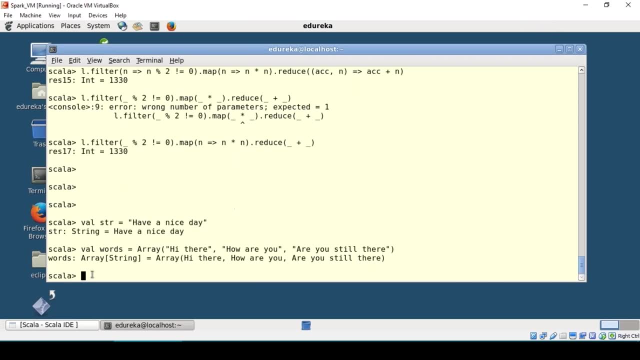 Okay, one more thing I wanted to show you is the flat map function. This is another very important concept, flat map function. So let me show you how a flat map is done. Okay, so say, for example, you know, here I have an array of strings. 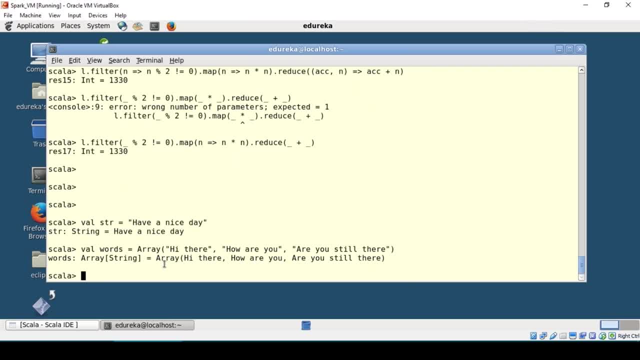 Okay, are you all following me Here? can you just look at the screen what I'm doing? I'm explaining to you the flat map function. It's a very important function which we are going to use in Spark. So that time you know. I don't want to repeat myself. 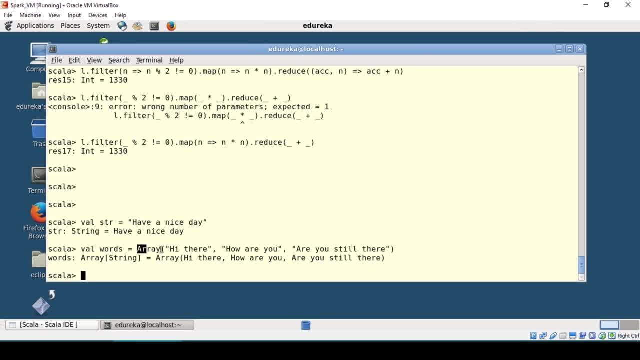 Please pay attention to what I'm doing here. Here we have this array. okay, It's an array of strings, So that means you know there are three sentences here. Hi there, how are you? are you still there? So it's an array of strings I have, and these are words. 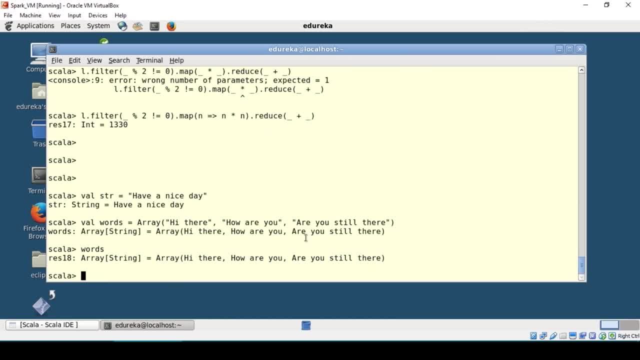 So these are, you know, three array of strings. It's an array of sorry, three strings. Now, if I call words, if I want to have, if I want to get individual words out of this, so what should I do? 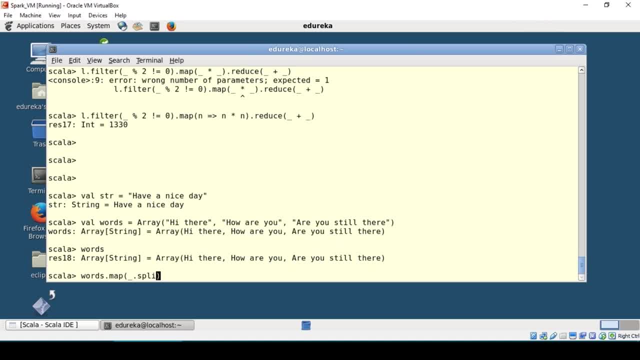 You know I should call the map function and what I do here is I basically split it based on spaces. okay, So what I do here is I take, you know, I take the individual sentences and I split it up based on the space. 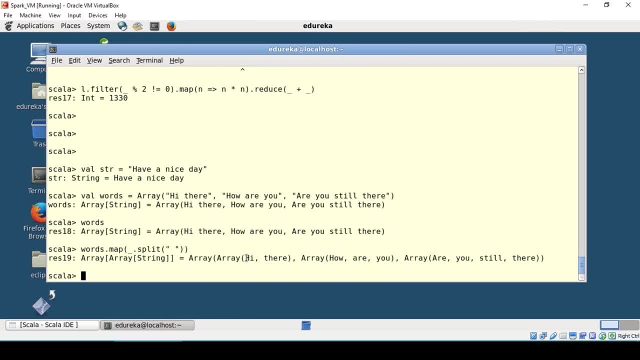 Okay, so then I'm going to basically, you know, get you know the individual words here. okay, So now you have the individual words, because previously they were sentences and now they are all words. Did you follow this line? what I did here? 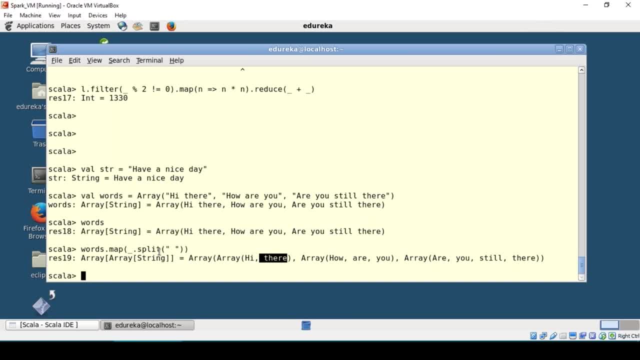 I took the map and split it. Can I have a yes, no, maybe, whatever got it Now here you will see a problem. The problem is that you know, now you have an array of array of words, okay, 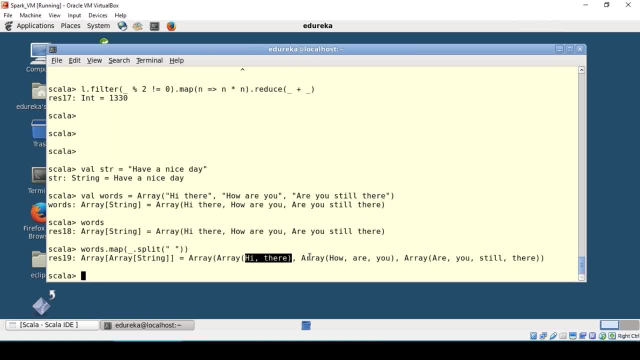 So, which is not desirable- You have an array and an array of array of words, which is what you don't want. okay, You want basically an array of only the words. So it has got an array. So it's something like this and if you want to visualize, 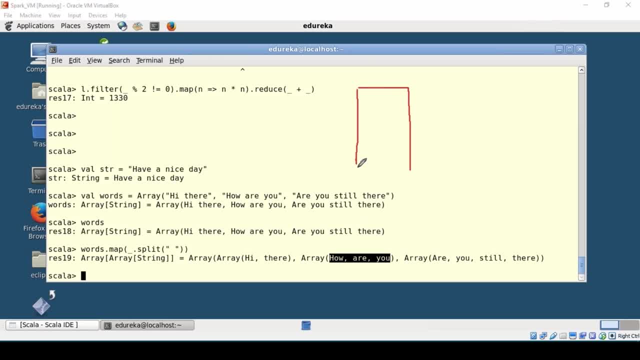 it is something like this: and you have an array, okay, And each cell is again an array okay, It's again an array of you know words. So the first one you know it's hi there. and again the second cell, it's an array of three words. 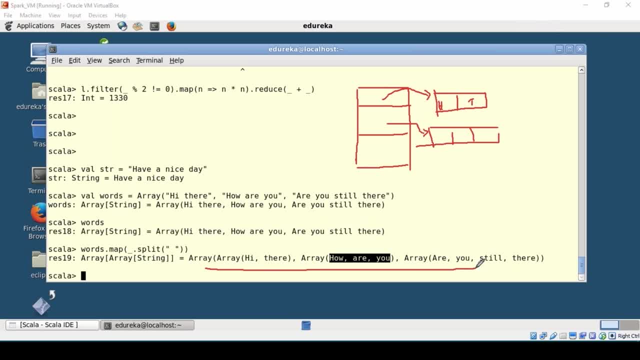 How are you Like that? it goes on. okay, I don't want this. So this is what I've got, but I don't want this. I basically want a single array. okay, I want one array with all the words, okay. 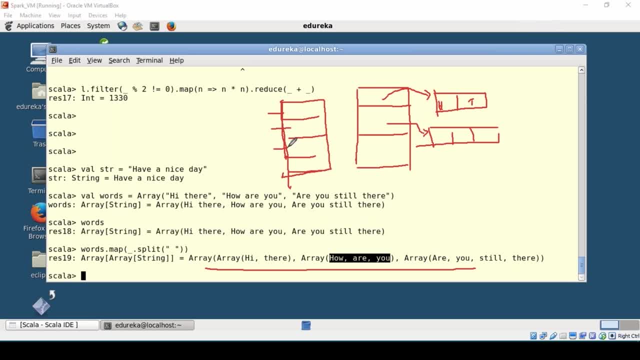 So that means: hi there, how are you, are you still there? So all will come, you know, in one array itself rather than as an array of arrays. So how do I do this? The way to do it is use the flat map function. okay. 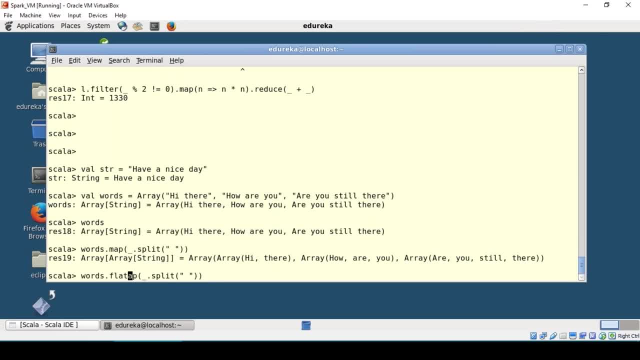 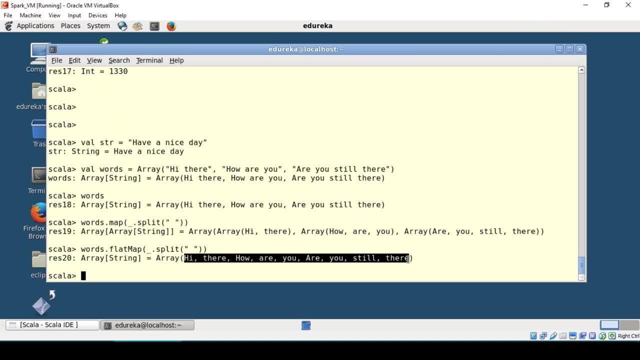 So it basically maps and then flattens. So the way to remember it is it basically first runs the map function and then it flattens the list. So now, basically, you get hi there, how are you okay? So this is basically how you have you know. 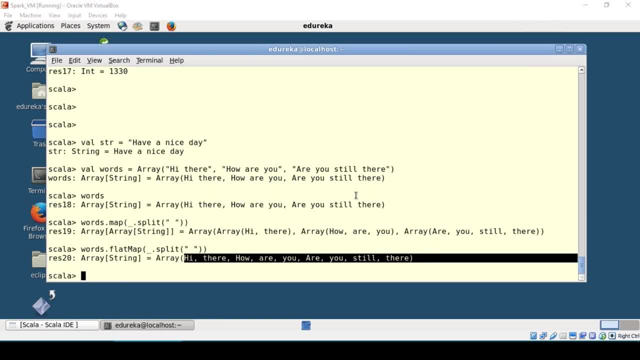 converted into one block of array. Are you all with me? Did you understand this line? Okay? so now, okay, some questions here Here. Rao is asking me that: okay, how do we use this in real time example? Yeah, first you tell me, Rao. 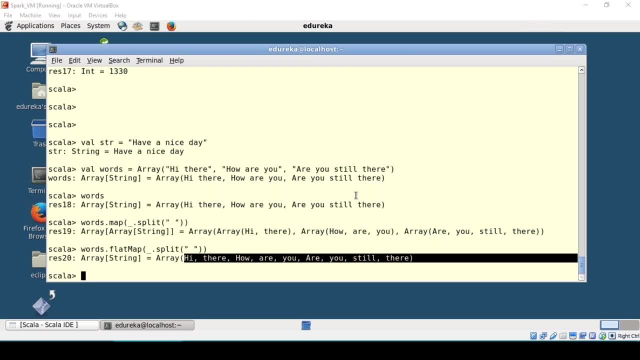 whether you understood this or not. That's more important. before I get into real time, or rather real life examples, Have you understood this? Okay, Shailaja is saying that we really don't need flat map for our example above, where there is only one array that we are getting. 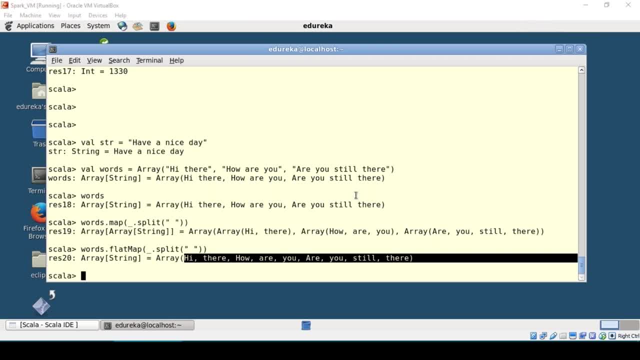 by splitting the string. Okay. Venkat is also asking: what is the real use? Okay, Ganesh is saying: we are getting music. I don't know what it means. Is it a metaphor, Ganesh, Because I don't hear music anyway. 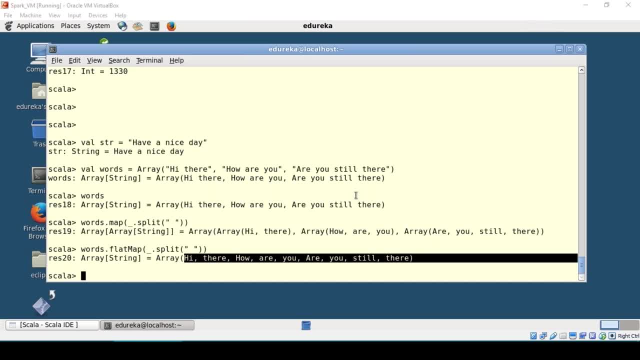 Okay. Rina is asking: is the space a delimiter? Yes, the space is the delimiter. Okay. Vimla is asking: the map function does it always return some type of collection? Yes, you're right, Vimla, The map always returns a collection. 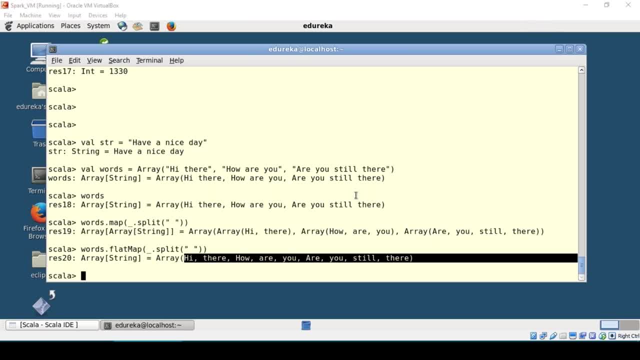 It applies the function to each individual element and returns a new function. Right, okay, concepts, you got it Now. okay, fine, now I'll just answer your Ganesh's and Venkat's question about real life applications. The thing is that say, for example: 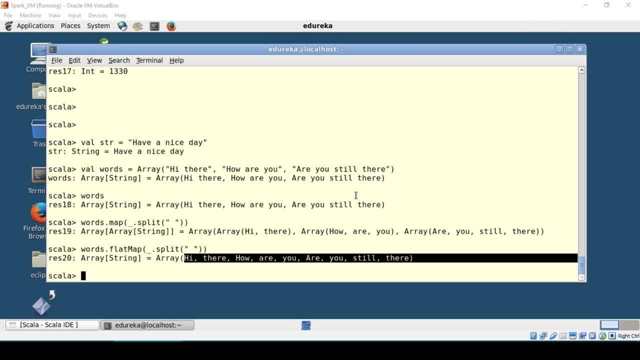 let's quickly get this. So say, for example, you are reading a file and you have read a file, and now what you want to do is: you want to do some analytics on this. Okay, so you have read a file and now what you want to do is: 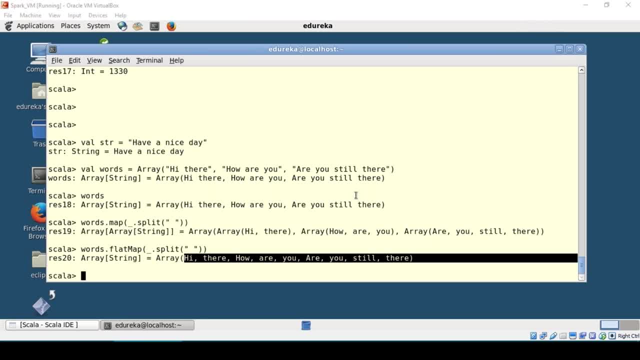 you want to do some analytics on this? Okay, so when we do Spark, you know I'm going to use this flatMap a lot, so don't worry about real life examples. You get fed up by seeing examples, But just to quench your thirst. 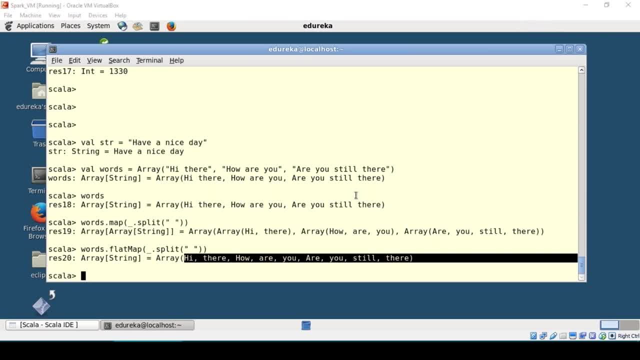 I'm just giving you the stuff here. Okay, Ganesh is saying that, instead of array, can we move to list? Okay, looks like he's allergic to arrays. Okay, Ganesh, so we'll move to list. Okay, so we have a list here. 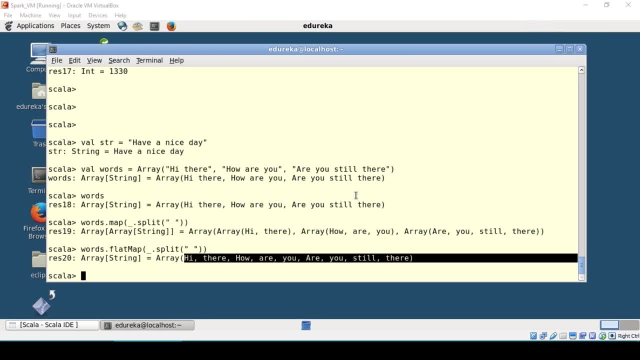 Okay, and not. what we do is even practical application. so we have a list. Now I can have words and then I can run a flatMap and on that I can split based on the spaces. So now you have a list of all the words. 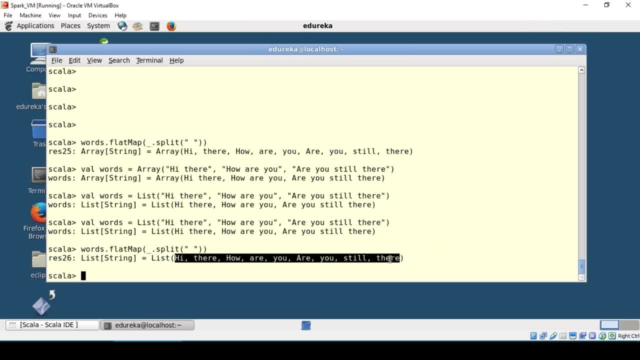 Now what I can do is: no, there will be some network latency in seeing the screen, so I change it to a list. and now what happens is, after doing the flat map, I can convert this words into tuples. So now what happens is: these are individual words. 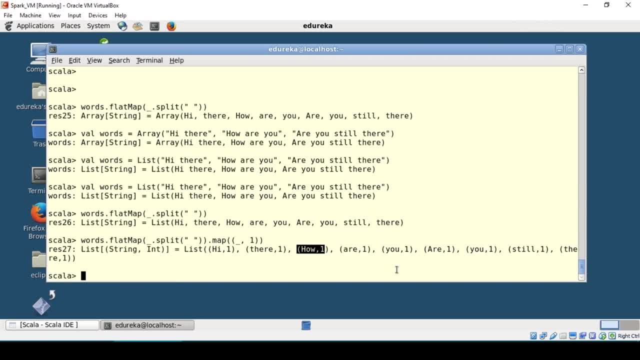 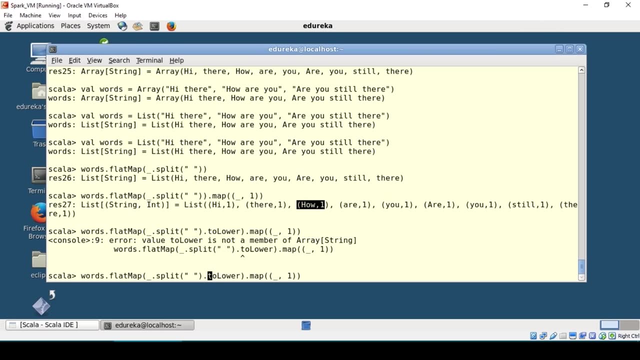 which are tuples. So, as you can see, these are all tuples. Now if I want to convert them to lowercase, I can actually run another map function just after splitting so I can say to lower. so sorry, Okay, I'll come to that a little later. 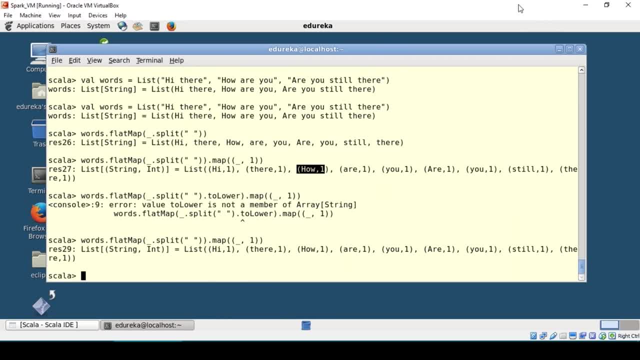 but just this step. have you understood this particular part what I'm doing here? Have you all understood this? Okay, so now what I do is I just convert everything to. I run another map function where I convert everything to lower. 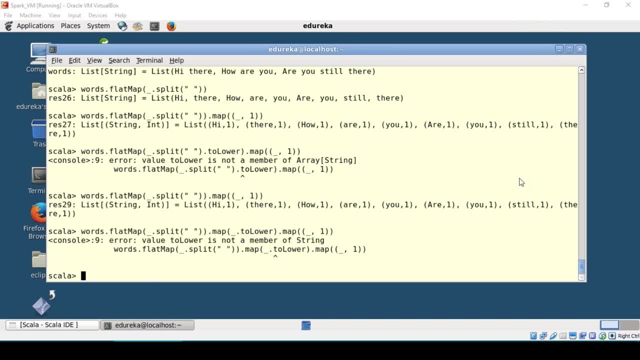 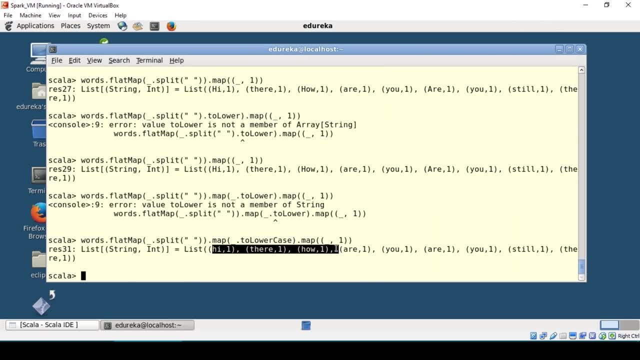 Okay. so what happened? There is no method called to lower, or what is it? Oh, I'm sorry, to lowercase, okay. So then what happens is you know, there's all these things are converted to lowercase and now you'll end up with tuples, okay. 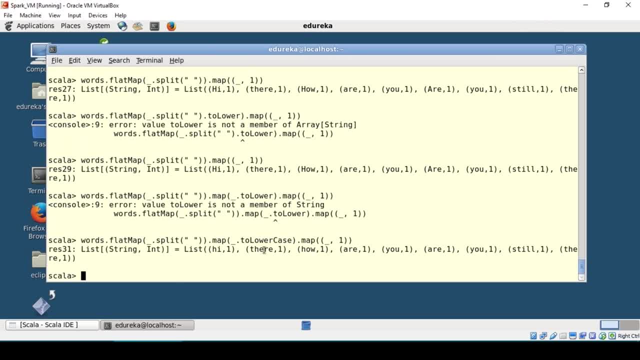 And then you can count up the number of words which are occurring and you can do analytics on that. and I'm going to do that more when I'm doing Spark tomorrow. but just to give you an example, say, for example, you read a file. 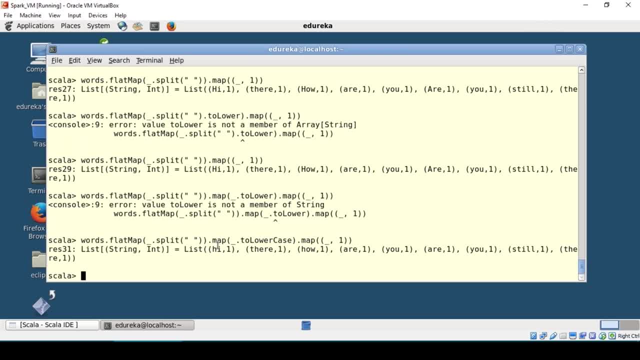 and say instead of sentences: you know, if these were files, then I could have read all the whole file and I could have converted this to a tuple, and then I could have accumulated all the similar words, all the words together, and I could have got the word count. 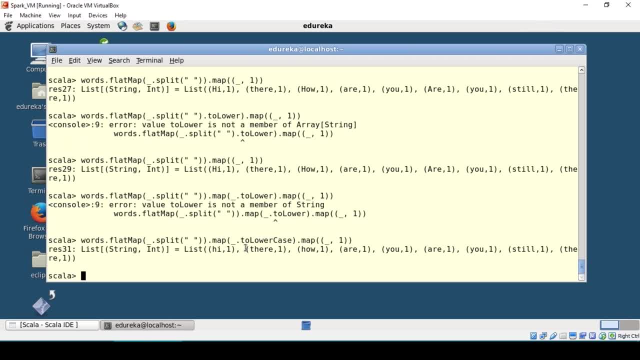 and after I get the word count, you know I can actually do analytics on that, so I can do all kinds of. I can find out how many words have occurred. how many times is how occurring, how many times is still occurring. 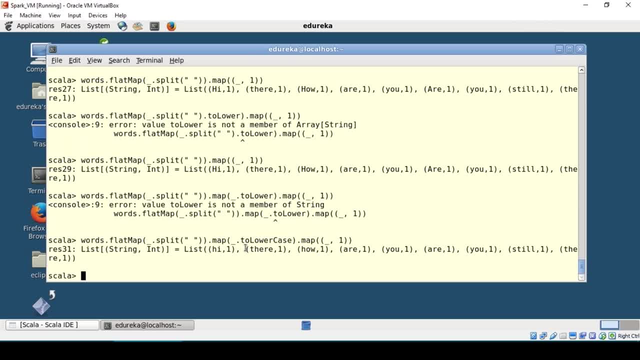 and all kind of, you know, real-time analytics. I can do. Clear Rao, clear Venkat. you asked that question. Yes, Ganesh, then you know I can do real-life operations. Okay, Shailaja is asking that how to combine the words. 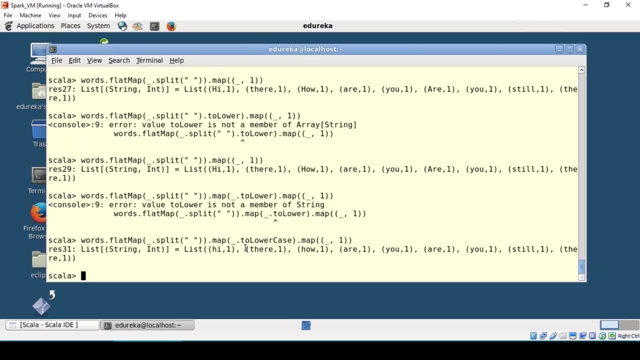 to count up. no, that I'll show it to you tomorrow. okay, you have to hang on so that I'll do it tomorrow. Okay, Vimla is asking that: how do we know when does the map function will return an array or list or tuple? 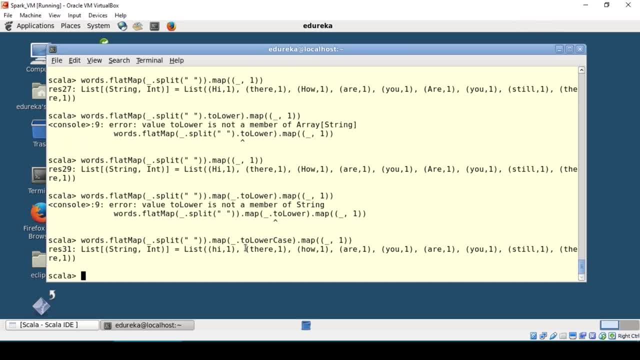 See, the thing is that you know whatever you're passing, that will be returned only okay. so the thing is that the original input of the words is list, so you know the map will return a list. If it had been an array, it returns an array.